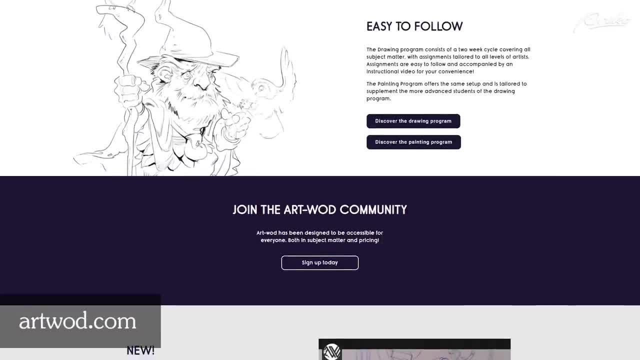 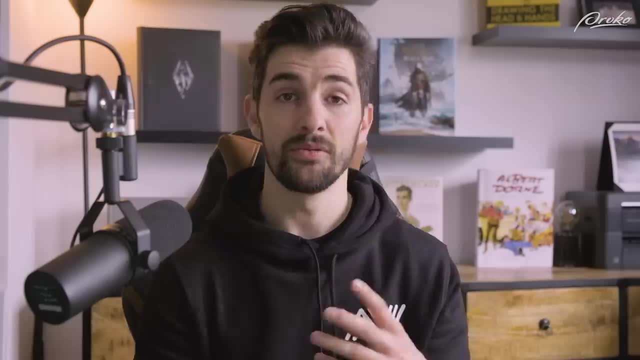 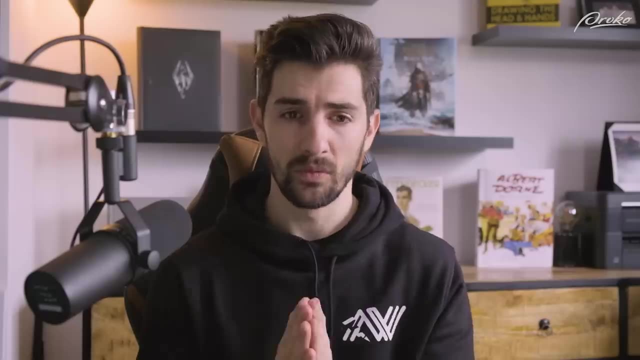 wanted to discuss with you guys today is the importance of structure in your artistic learning, Primarily about structure in your drawing and painting, but also a little bit about structure in the mental aspect of being an artist. Primarily, what I wanted to discuss is what I call a six. 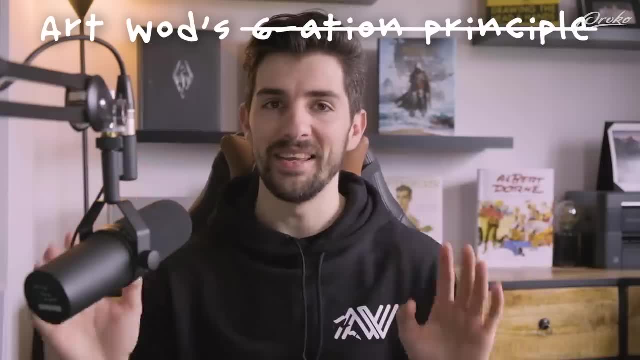 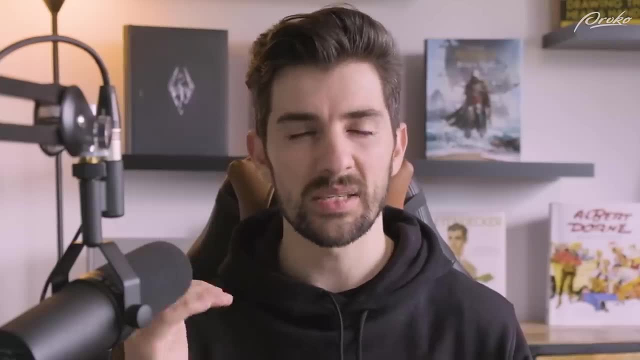 Asian principle, And don't quote me on that. I just made it up to sound a little bit smarter and make this a little bit more clear for you guys. But I want to discuss six principles that can help you understand better how you can come up with the right principles for your art. 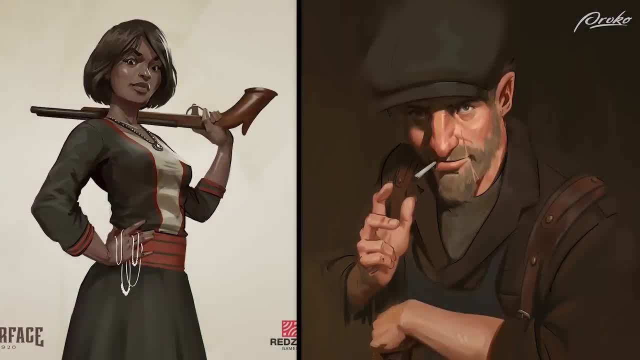 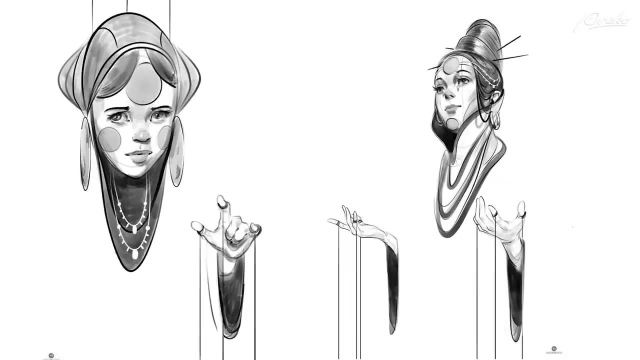 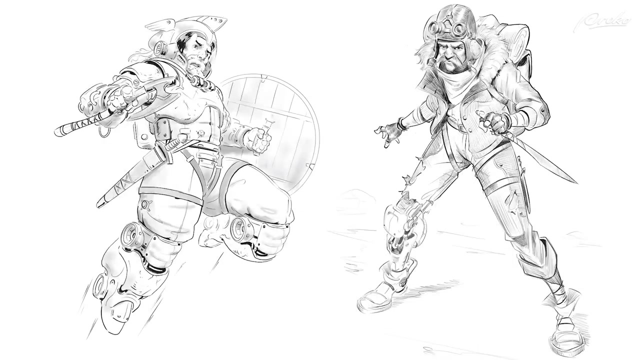 With more complex drawings, where I feel that a lot of beginners, intermediate artists- they tend to fall into the trap of learning the very basics and then quickly moving on to very complex shapes. You see this a lot when people just they learn the basics of perspective. 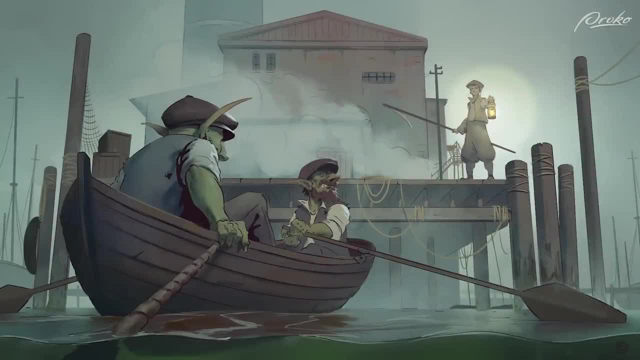 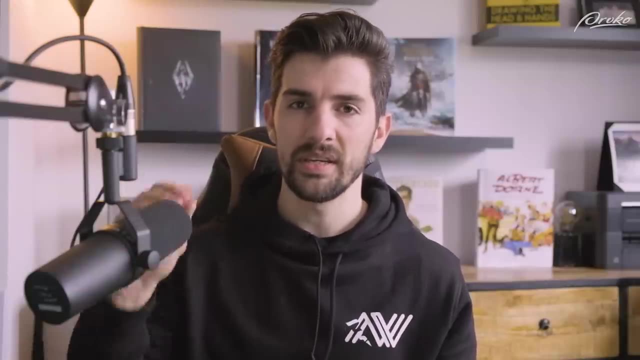 and then quickly move on to complicated scenes or figure drawing or whatever. And now that is important. of course, you know challenging yourself, But I feel like there's a really nice setup that you can use, which I use in my program as well- that can help you better. 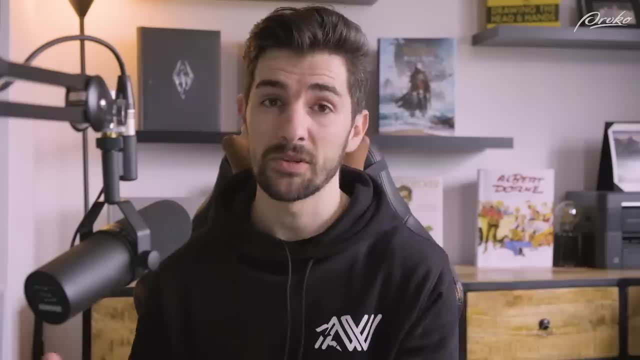 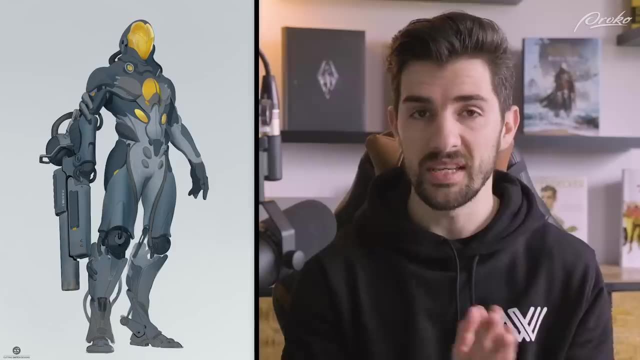 understand how you can come to these nice and complex results that you see from a lot of professionals, especially people drawing from imagination, Because my focus is in that world of concept art and you know, coming up with new ideas, interesting things, And you know. 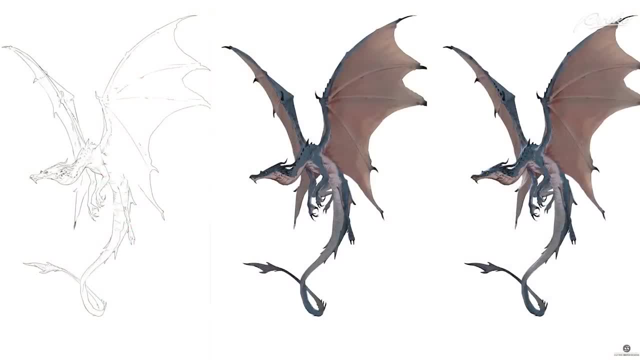 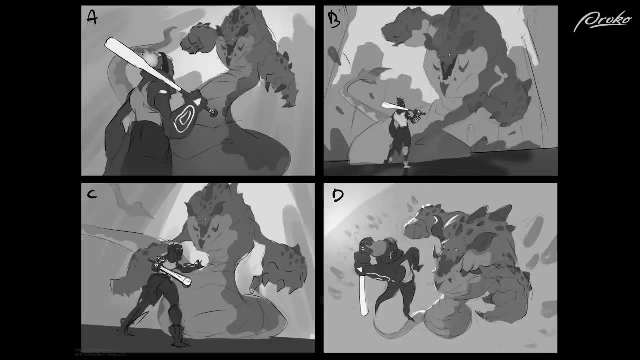 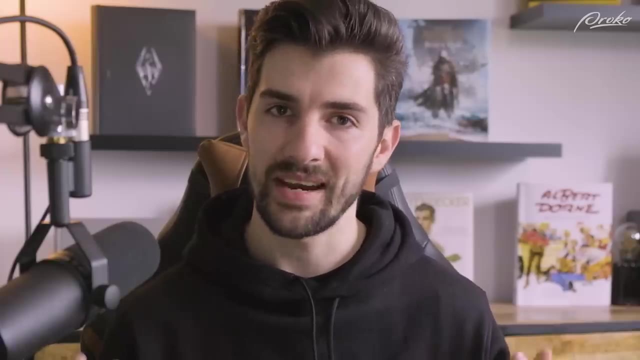 design is a big part of it, And if you can internalize a lot of complex ideas, things that you see, into more rudimentary yet complex shapes or mannequins, it gives you a nice tool to create your own things. So the six Asian process that I want to talk about today, the first one is: 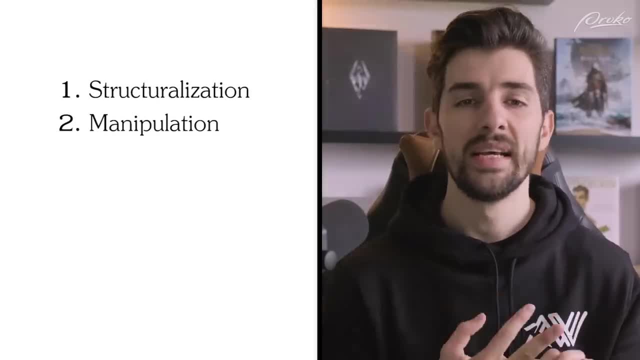 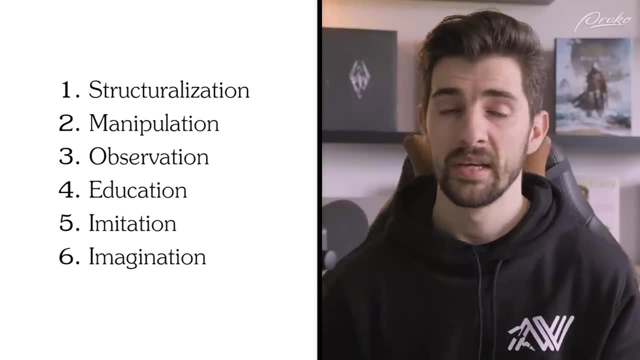 structuralization. The second one is manipulation, and then observation, education, imitation and, lastly, imagination. So, without further ado, let's just get started. So, when it comes to structuralization, I'm going to talk about the six Asian processes that I want to talk about today. 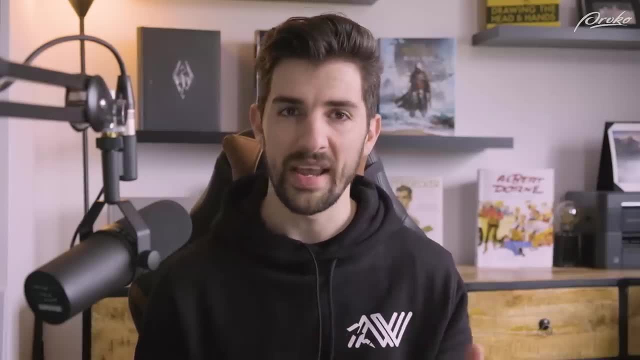 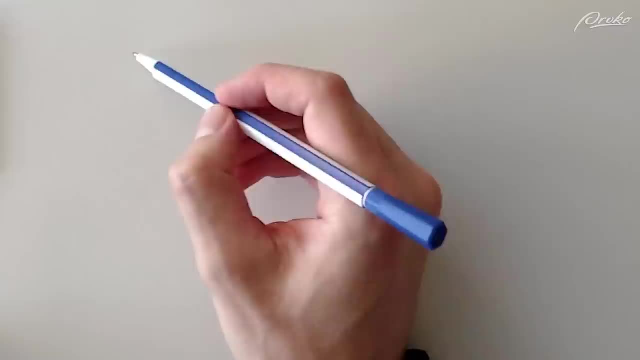 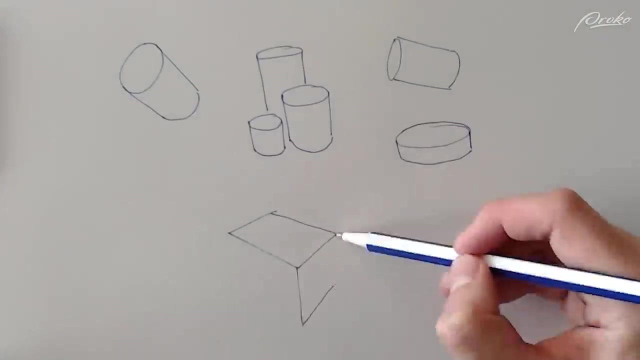 This is the most straightforward for anyone. It is that very basic, rudimentary aspect of just learning to draw the simple shapes, cones, spheres, cylinders, boxes, and kind of creating that spatial awareness, not only being able to draw a box in one point or two point or three point. 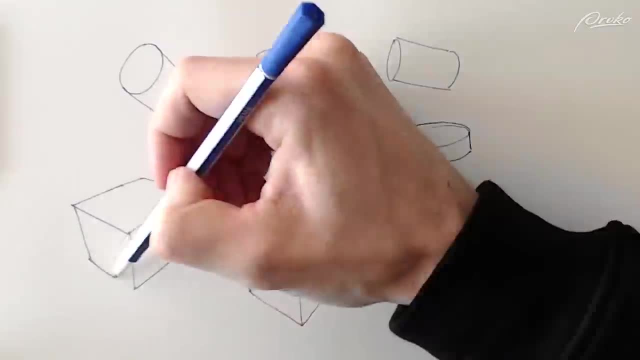 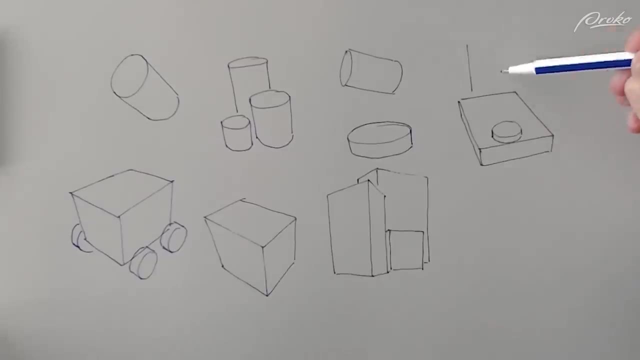 perspective, but also learning how to intuitively draw a box in space and draw multiple boxes grouped together, draw a cluster. And then the last one is the three-point perspective, which is the three-point perspective, which is the structure of primitive shapes together and just learn how to do. 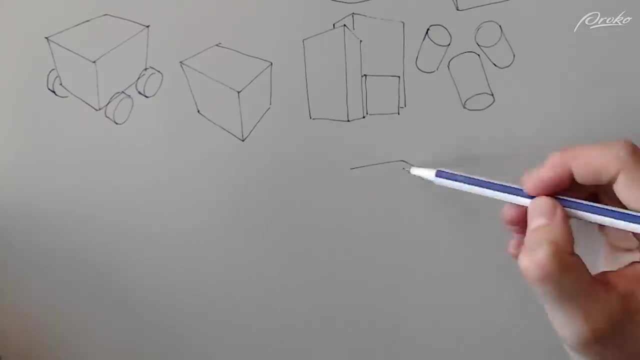 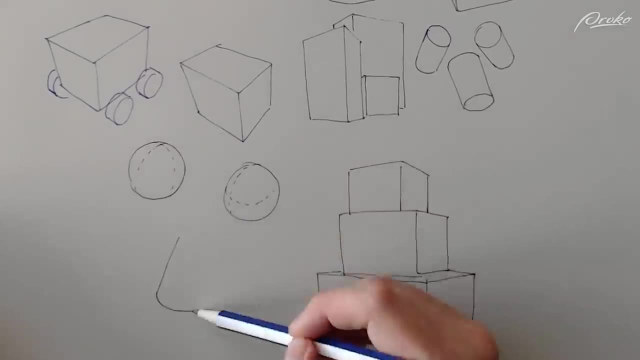 that intuitively. Now, of course, you do need to learn the rules of perspective, maybe even camera angles and how they relate to perspective, to be able to do that, But I feel like that's a really good starting point: just to draw simple shapes on paper and get a good sense of spatial awareness. 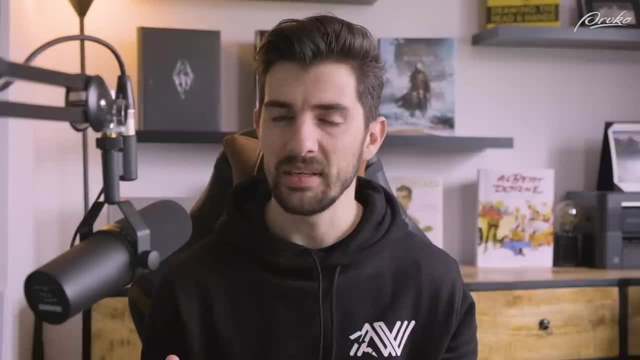 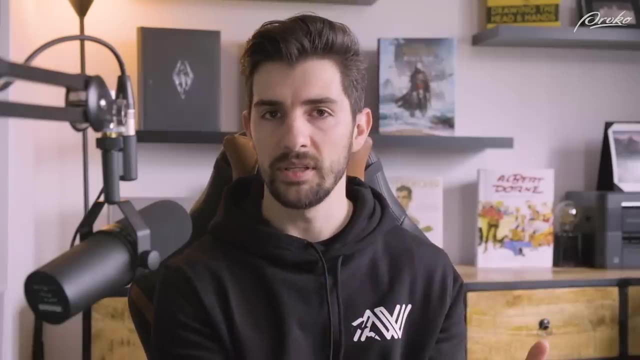 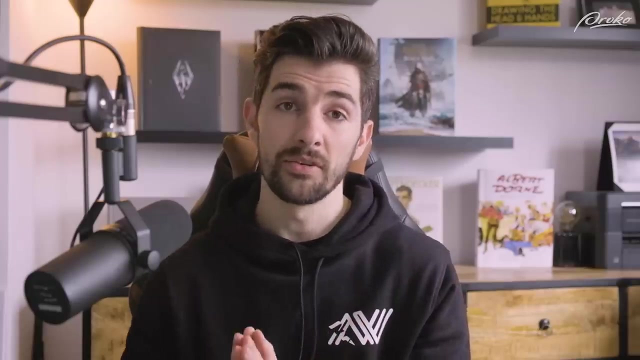 because that's what it's all about. In order to create anything believable, especially when you want to communicate something to you know further down the pipeline, especially in the concept art industry, it's all about communicating properly, And a lot of the times that means communicating your designs to the 3D modelers. 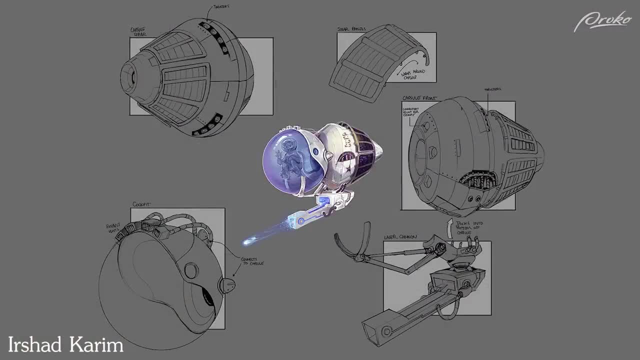 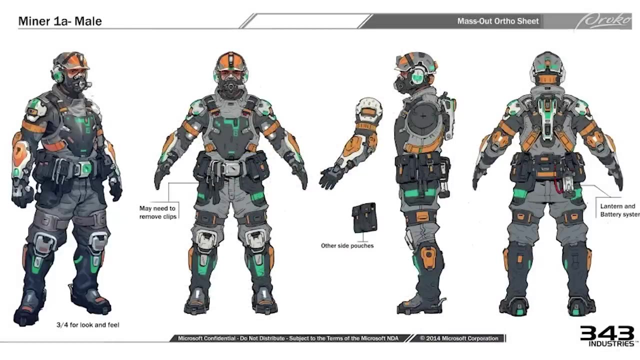 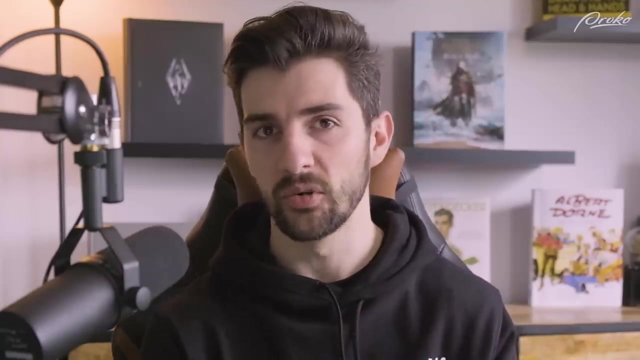 or the animators or environment artists or just the art directors in general. That sometimes, or often, requires that you create a good sense of believability in your designs and that everything feels readable as it should be. Now, that's the first step. It's pretty straightforward. 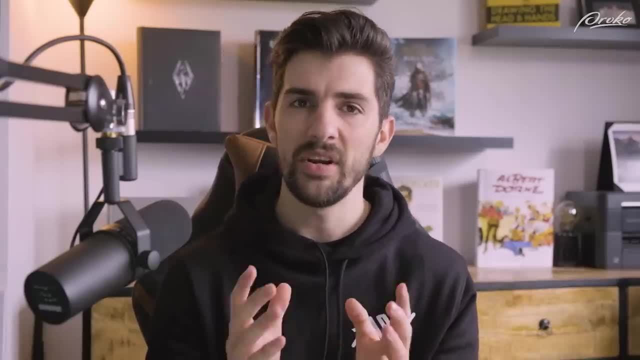 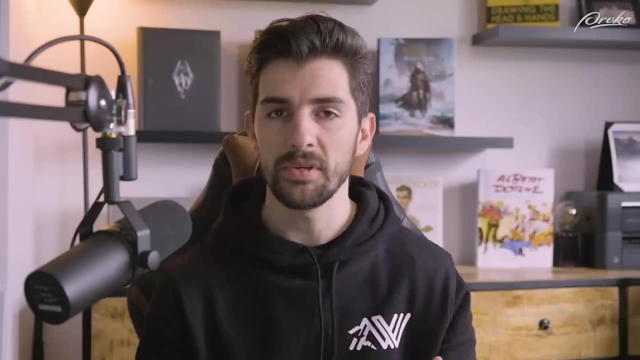 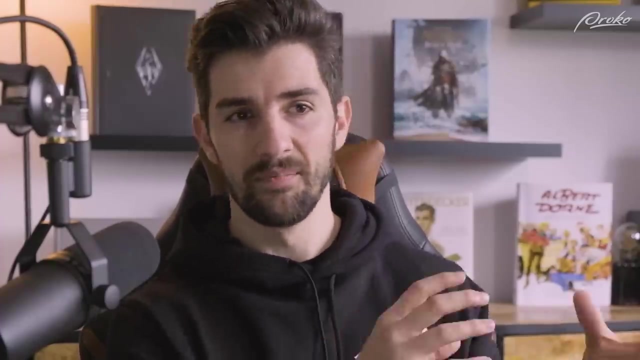 And moving on is one of the steps that I feel is very, very often overlooked, And this is what I call manipulation, And in broader terms, it's shape manipulation, And so there's a high number of ways that you can manipulate a shape, And a lot of you have probably seen excerpts of how it's done, But I 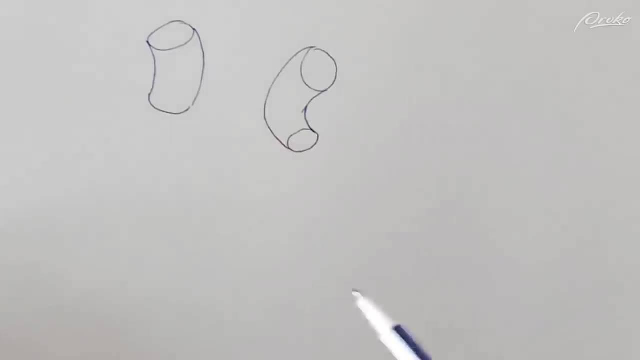 feel like it's very often overlooked in people's artistic training. There's hundreds of ways to manipulate a shape, but I'm just going to go over a few of them. So one of the ways that you can manipulate a shape is by taking the primitives and then learning how. 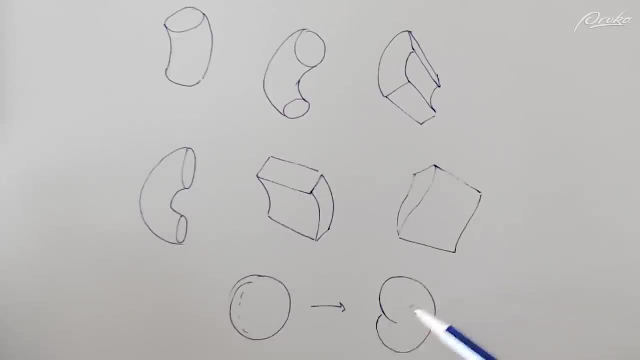 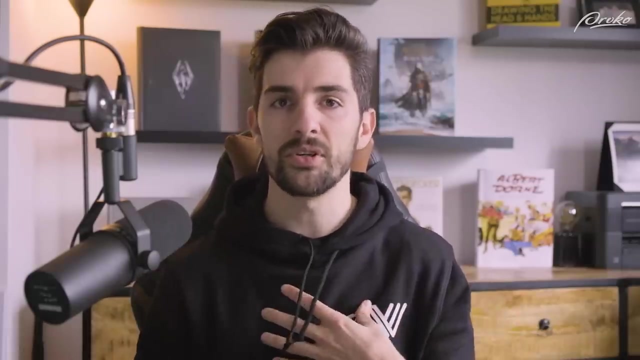 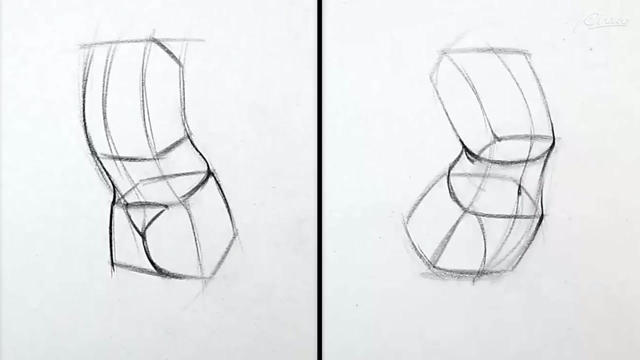 to bend or twist them. You know, this is a very basic one. It's one that you can also see, for instance, in the Proko videos. when it comes to simplifying the torso is: just use the beanie, right. The beanie is basically a bent sphere and things like that, or a box that is twisted, And 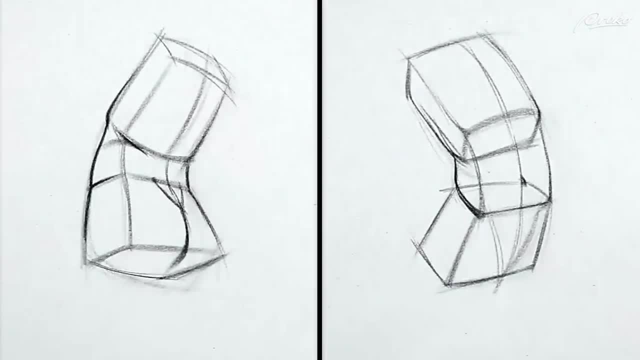 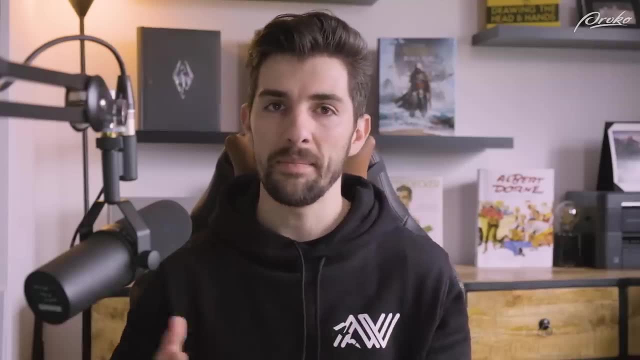 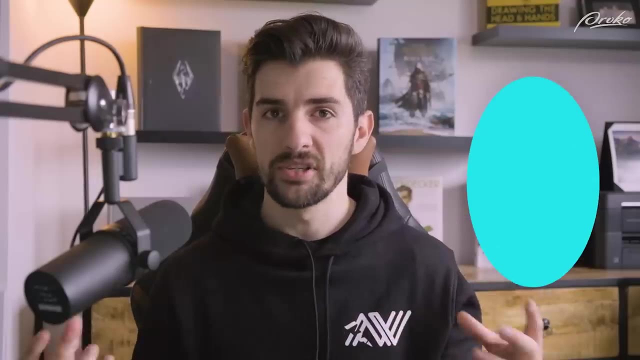 if you can already learn to manipulate simple shapes, you'll have a much easier time to then come up with more complex shapes. So I feel that you can really take a step-by-step approach in this process. Another manipulation, for instance, is learning how to squish and stretch shapes. You 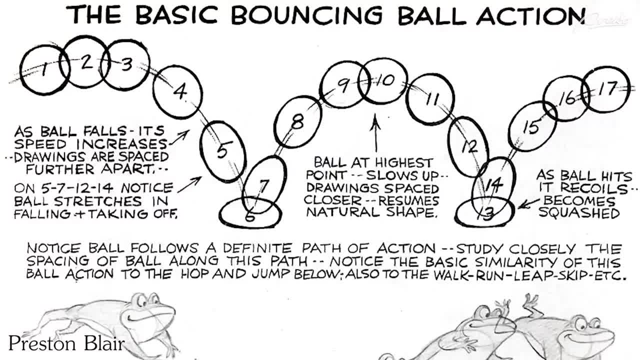 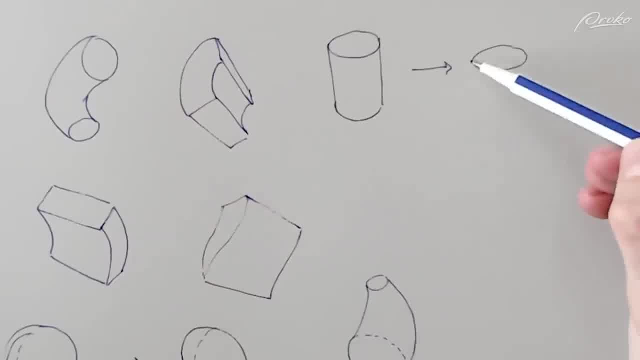 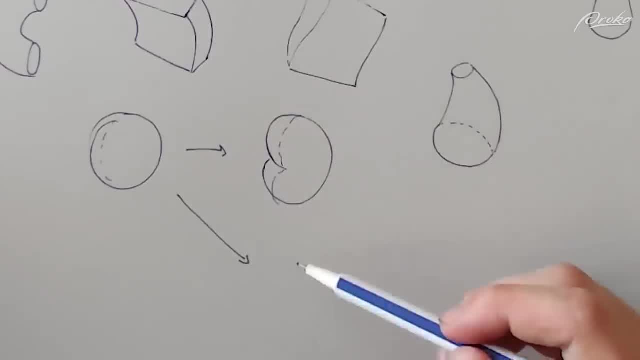 often hear about this in animation, where it can really help you create a gestural feeling in your drawing, or it will just create a better sense of movement. So learning how to just take cylinders, boxes, cones, whatever, and learning how to stretch them and squish them will give you a lot of. 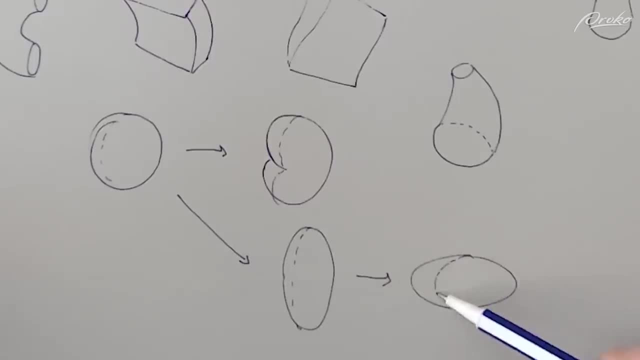 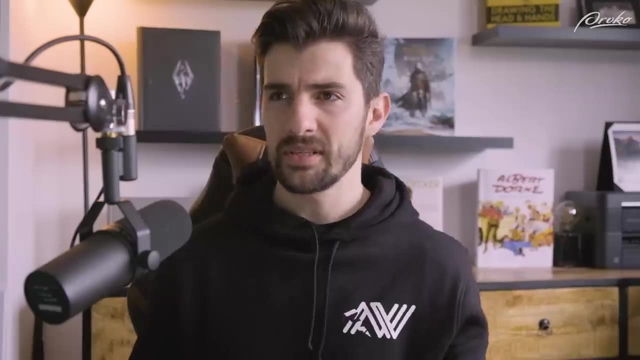 more freedom when you're looking at more complex shapes, on how to interpret those shapes as well. Another manipulation, for instance, is learning how to manipulate the contours. Now, this is something that I haven't seen too many times, or people you know put in a different jacket, or 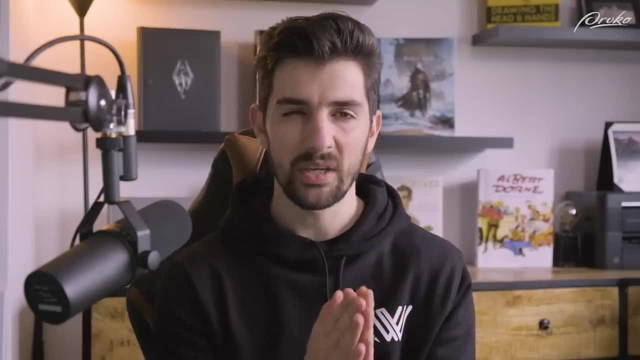 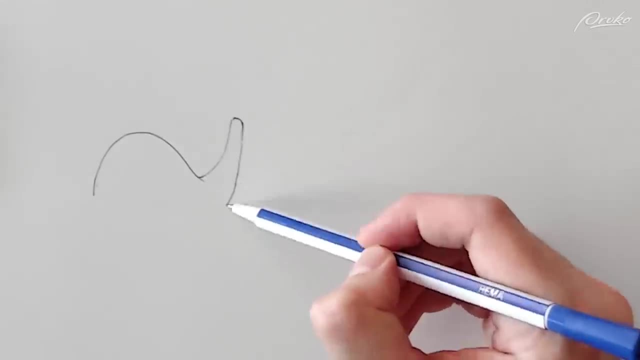 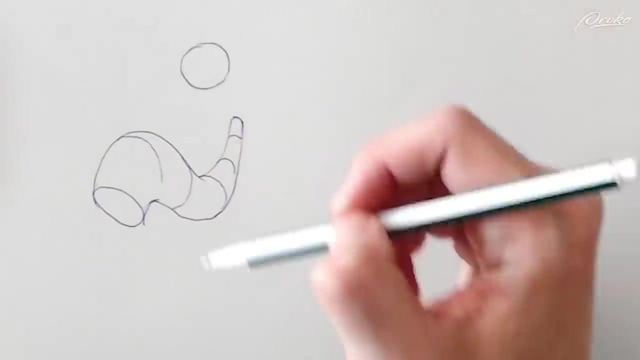 whatever, But learning to manipulate a contour will really, really help you when you're looking at more organic shapes. So, for instance, if you take a cylinder, that's being manipulated, you know, by bending it for instance, the contour of the cylinder is just a circle, right? So it's a circle. 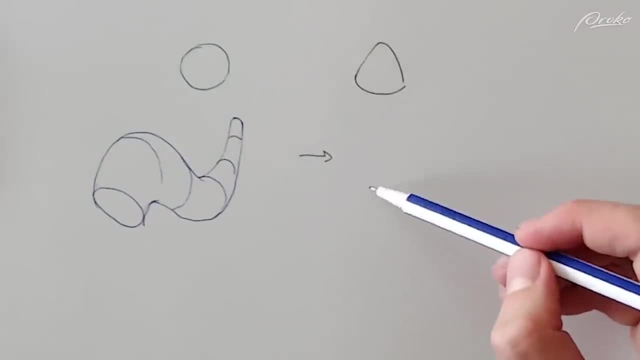 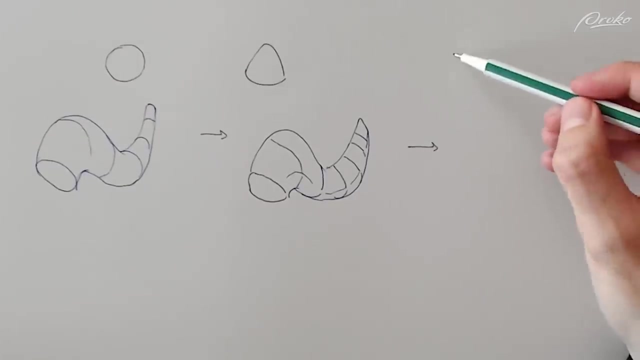 going around and around. Now, if you can learn to manipulate those cylinders, for instance by changing that circle, which is the contour of the cylinder, changing that to a triangular shape, or changing that to something even more organic and then trying to draw that shape again, you can come. 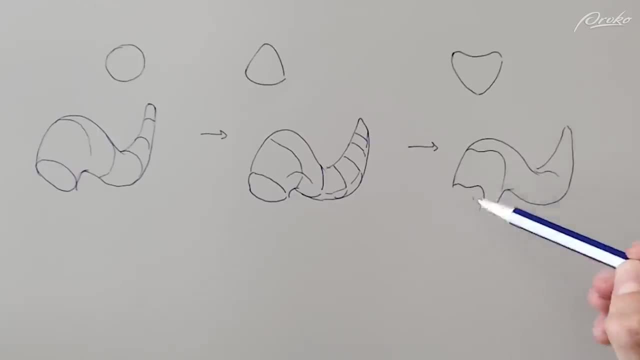 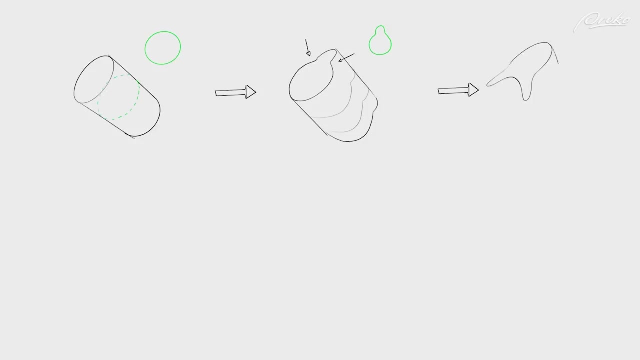 up with. you know very interesting shapes, but also shapes that are much, much more representative of real-life things. Think of the horns of a ram or a goat, for instance. This shape can look very intimidating at first, but if you think about it as a cylinder first, 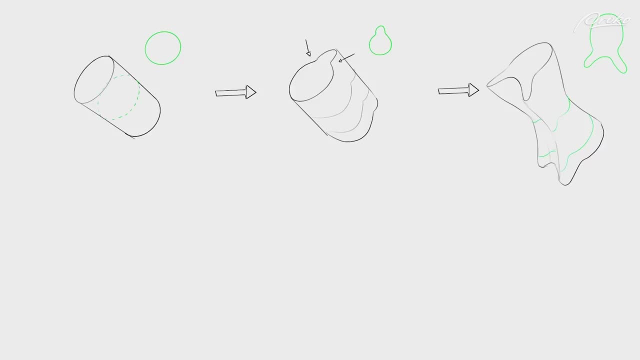 that is just being bent and twisted, and then thinking about how that twisted cylinder is being manipulated, the contours are being manipulated. then it makes a lot more sense and it's also easier for you to either stylize, exaggerate or just replicate. 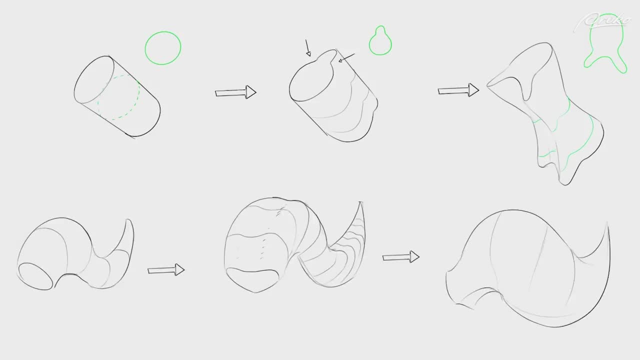 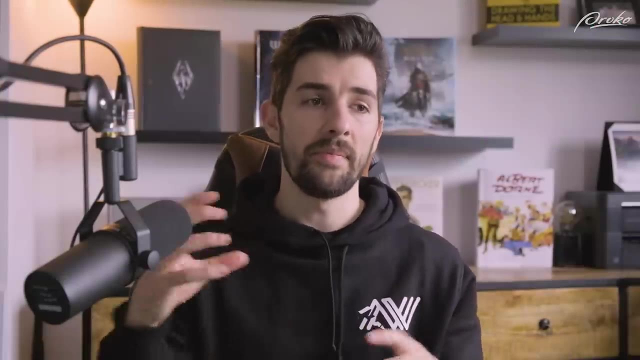 it, And that's something that I think is really, really important, And I think it's really really important to try to replicate what you're seeing. So contour manipulation is a really, really big one, I feel. Also, when it comes to, you know, drawing dragons, for instance, dragons are an amalgamation. 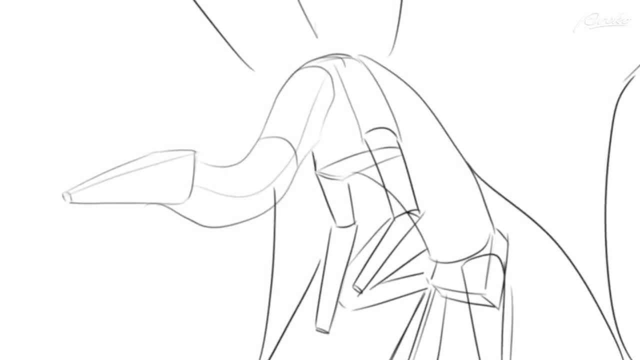 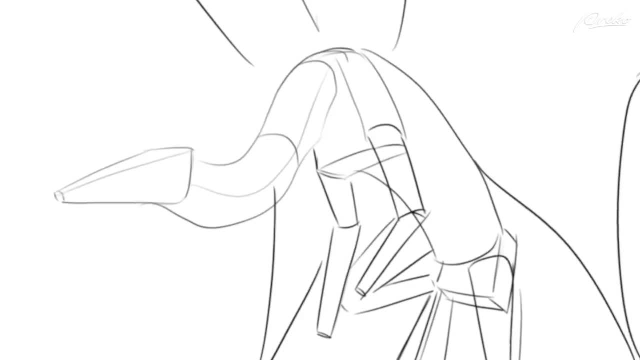 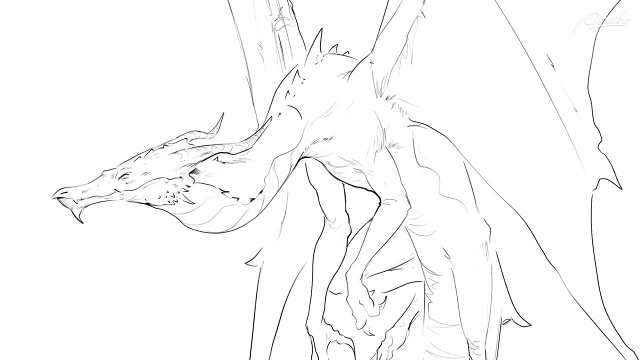 of different animals. But if you look at, for instance, the neck of a dragon, you can interpret it as just a cylinder, which is the very standard structural approach. But then if you think about how you can manipulate the contours of that cylinder by giving it, you know, a cooler contour, 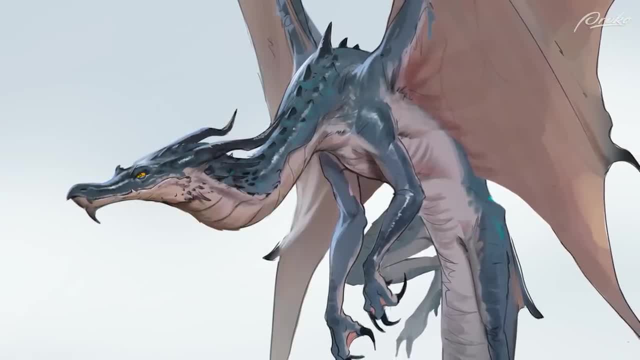 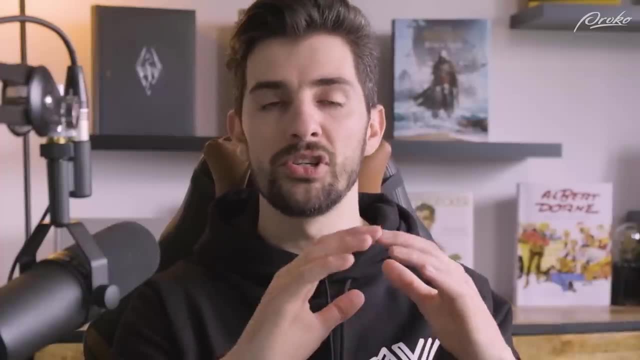 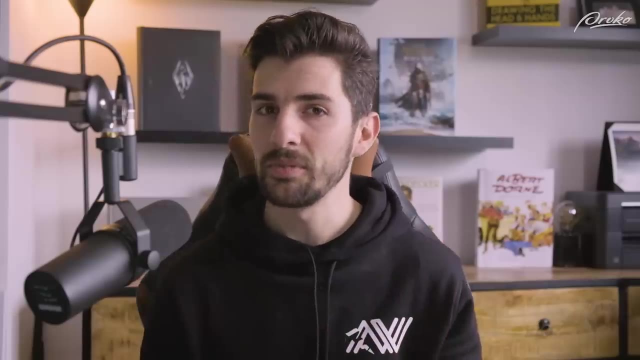 cooler silhouette, cooler you know section, so to speak. you can come up with a lot more interesting shapes And basically you're still working with a very mannequinized shape, but you're just manipulating its contour to already have a much more organic feeling. So again, contour manipulation is a very 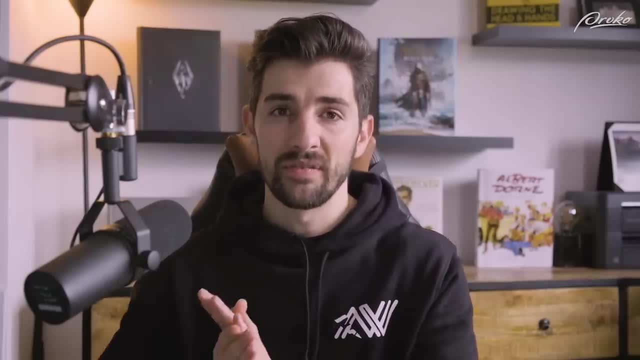 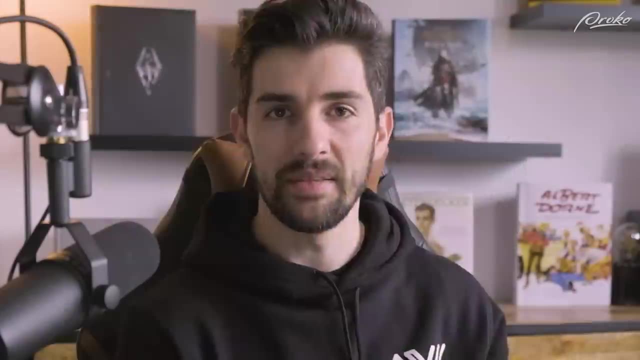 very big one, And that's why I advocate so much of learning how to manipulate shapes in its simplest form before you do it on more complex shapes- And that's what I was talking about earlier as well- a lot of people will learn the basics. 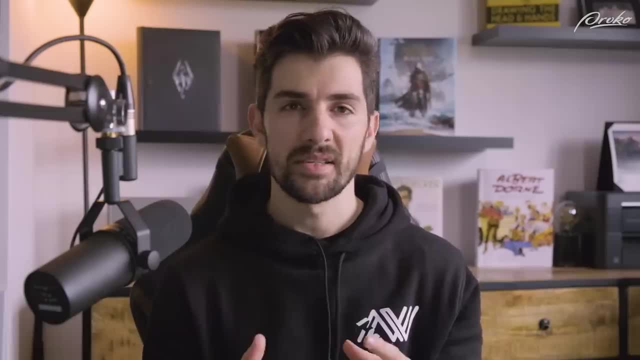 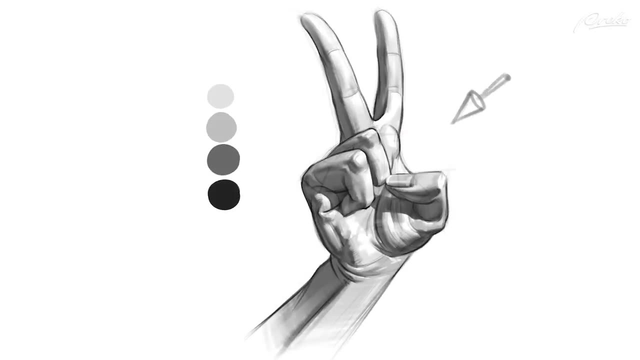 and then they will immediately jump to a very complex subject, Whereas if you first jump from the simple shapes to making those simple shapes more complex, that will help you understand the more complex subjects that you'll be looking at later a lot better. And then, lastly, I 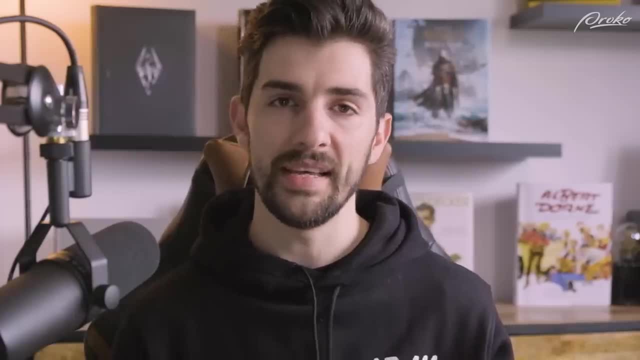 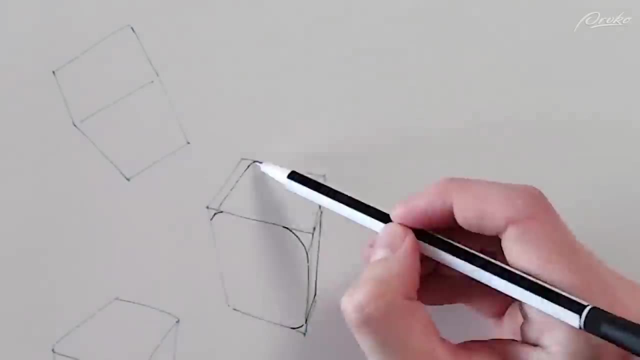 think another really cool shape manipulation is the manipulation of edges, And that's primarily when it comes to boxes and cylinders. So you know rounding off edges or beveling edges, things that you also see in 3d, for instance. if you can start to learn. 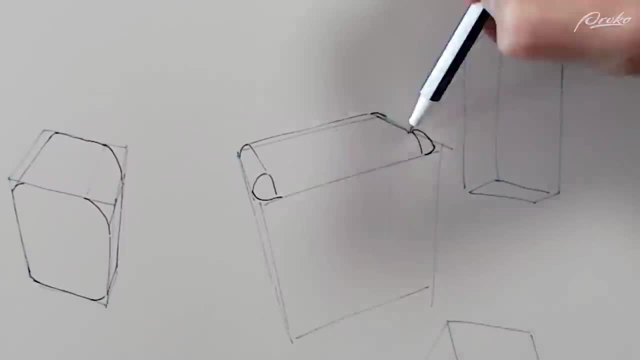 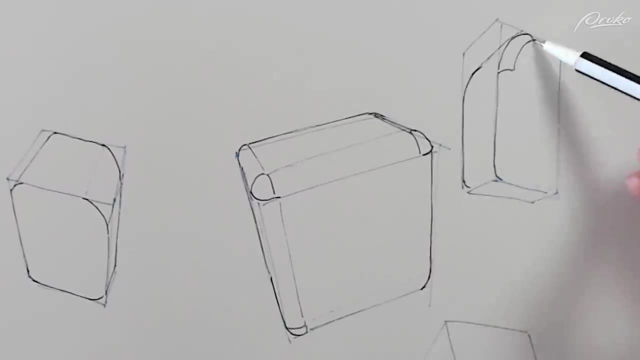 this on a basic or simple basic shapes. it will be a lot easier for you to understand more complex shapes, especially in hard surface subjects. for instance, if you can learn how to round off the corners of a box, you will have a better or an easier time understanding how hard surface things. 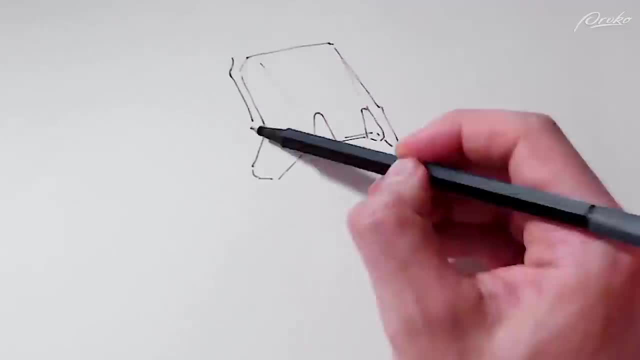 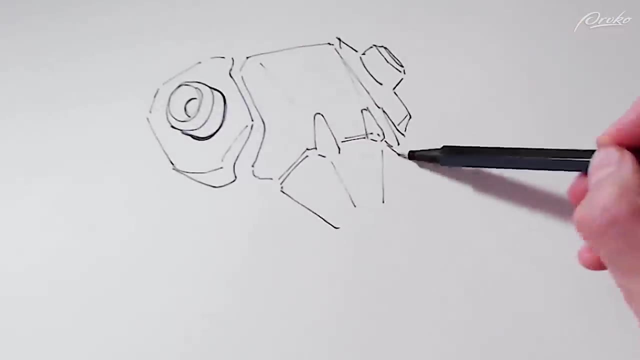 like mech designs are being created, because basically it is the same principle. it's just a little bit more advanced when it comes to the way they round off that boxes and the degree in which they do it, or you know, the asymmetry in which they do it to create more interesting shapes. but again, 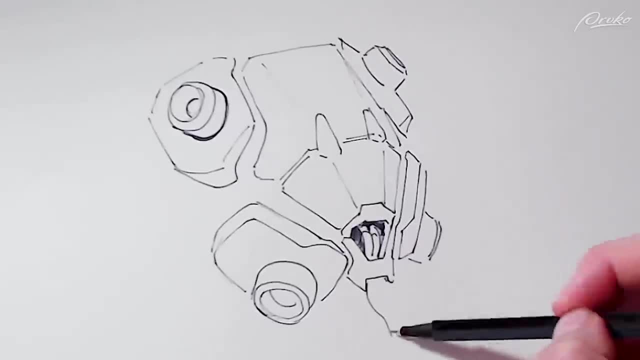 the principles are exactly the same. it's just taking a primitive shape and then rounding out the corners, or subtracting and adding new shapes that are still, you know, have rounded edges or whatever, or feel a little bit more organic to create that interesting shape. and i think that 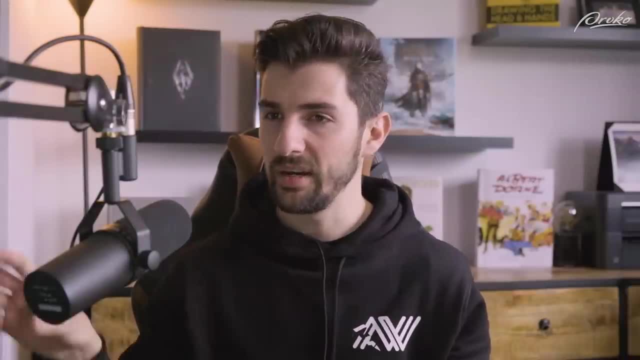 if you can, if you can look at a complex shape and you can look at a complex shape and you can look at a complex shape and you can look at like that which I teach a lot of my students is: look at something and try to analyze what you're. 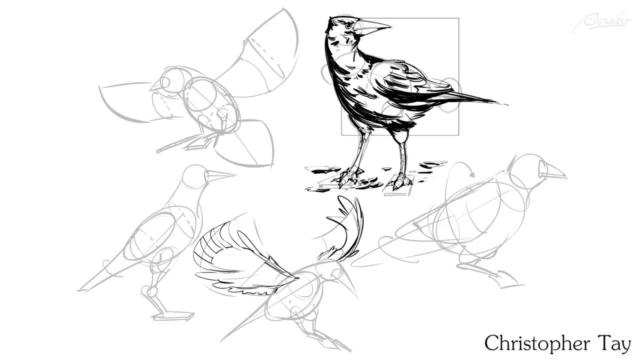 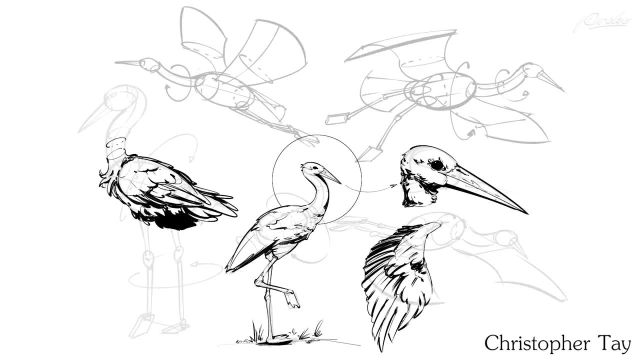 actually looking at like what's being manipulated, not just blindly copy what you see. try to understand what you see. I think that's a really crucial part, because when it comes to anatomy or draw or the human figure, it's uh, it's almost a given, like everyone understands that if I want 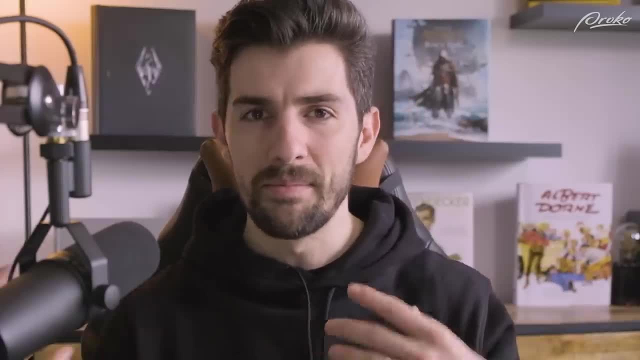 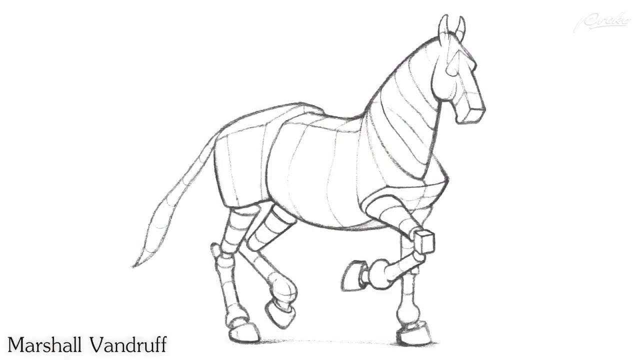 to be able to draw figures better, I need to understand the mannequin, and even the complex mannequin or the bridgeman mannequin, but when it comes to other subjects, I feel like it often gets overlooked in terms of understanding what you're actually looking at and you know with these. 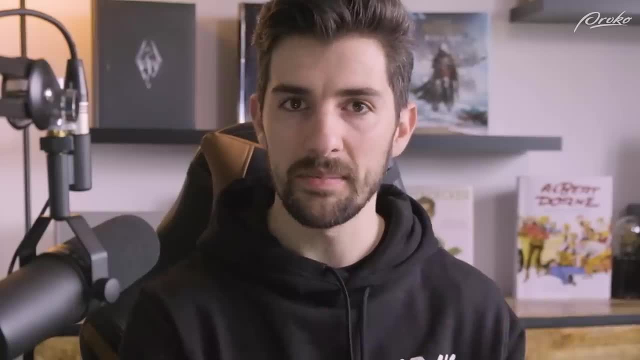 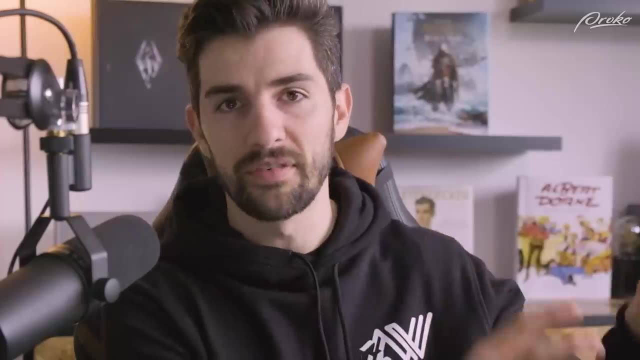 manipulated shapes or just learning to manipulate simple shapes, you'll have a lot more in your tool bag to then look at other shapes, random in life, or designs from your favorite artist, and understand like, okay, this is what it's being manipulated, what they're trying to do with the 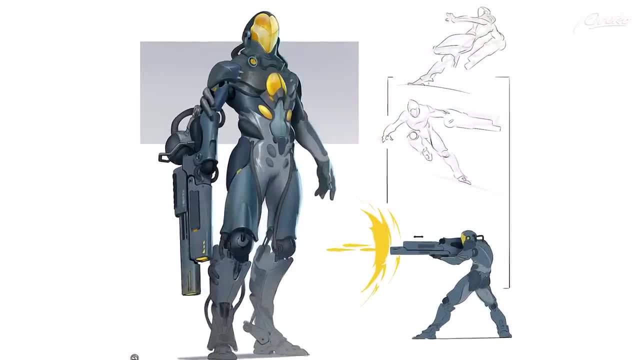 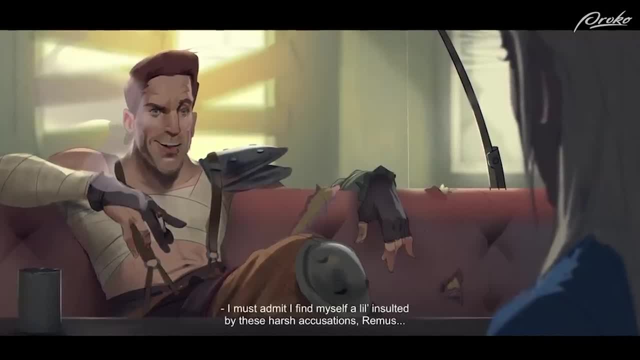 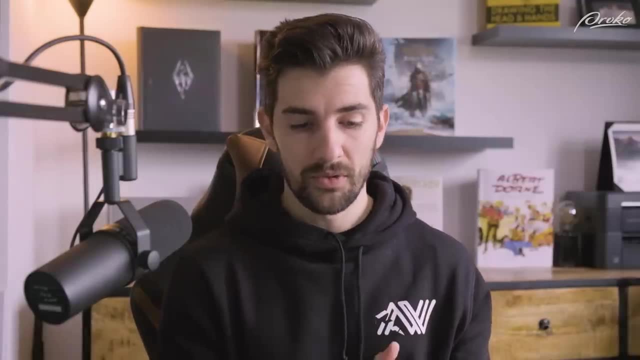 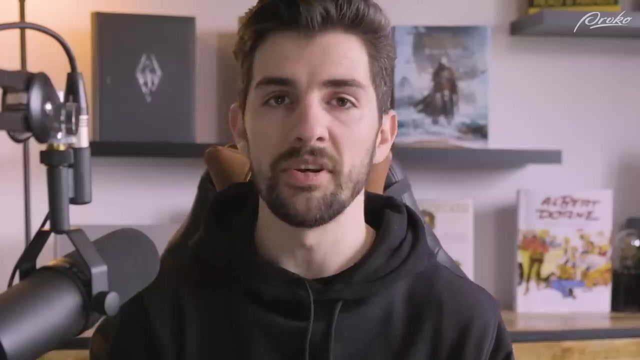 and I highly recommend that you try it on simple forms first, before you move on to complex shape, and then, thirdly, is observation. so the way I put up this six-step process is that everything builds on to the last step or its previous step. so that means that you know we have the 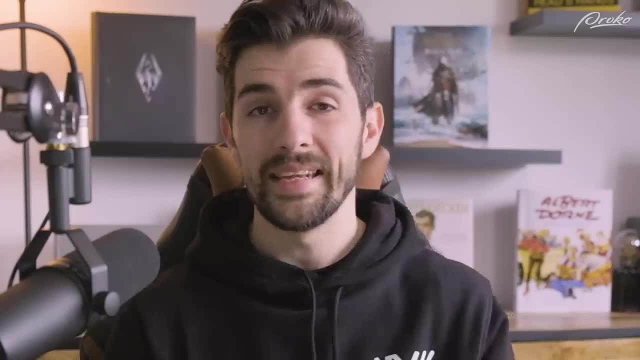 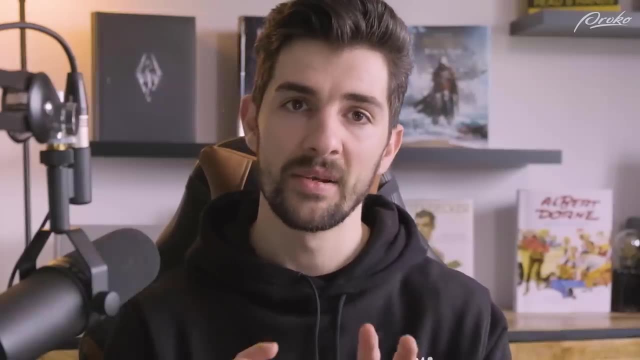 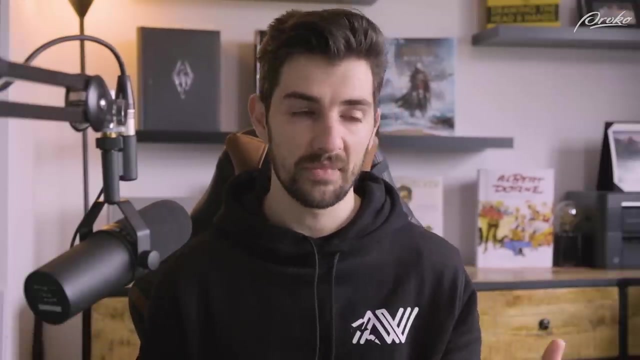 structural ization and then you can manipulate the structure and then in the observational part we can use those manipulated shapes and see how we can mannequinize what we're looking at, what we're basically observing. so, for instance, that means if we're looking at anything like an animal, whether that's a squid or, you know, an alligator or even 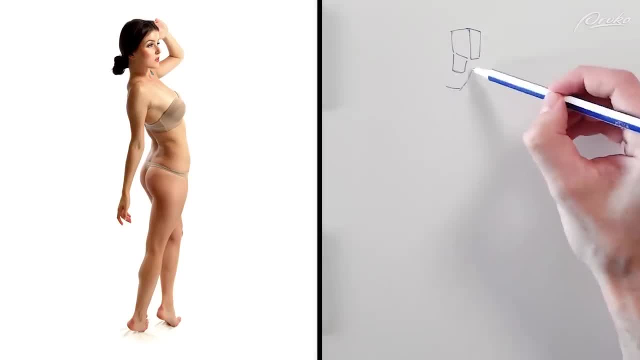 a human being, we don't necessarily already need to understand everything about what we're looking at, so that means that we don't need to first educate ourselves about the anatomy or what makes up that subject. we can just simply observe what we see and through our spatial awareness. 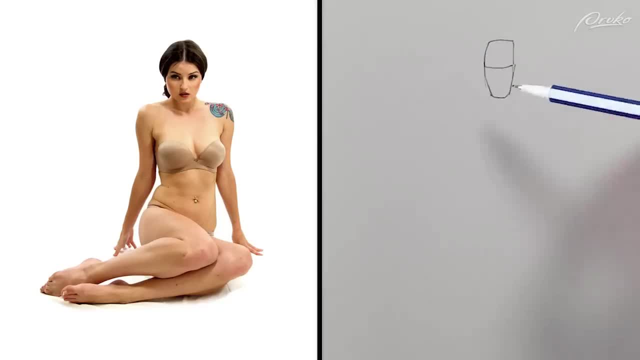 that we got from the structuralization, from, you know, our knowledge of perspective and organic forms and for manipulation, we can sort of already come up with something that resembles what we're looking at, and i think the crucial thing about this is that it gives you so much more power when it comes to making things from imagination, because 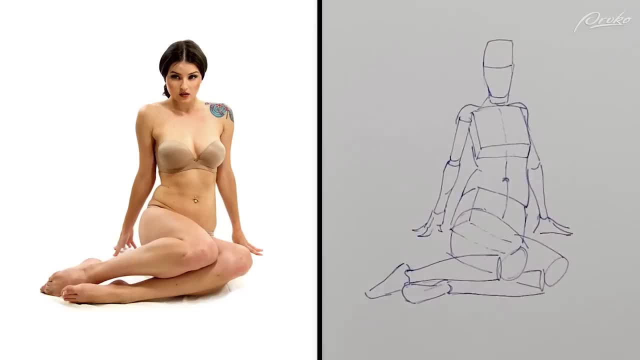 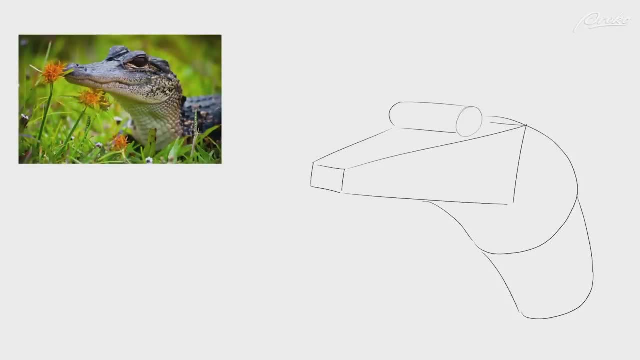 it's virtually impossible to remember everything when it comes to technical detail, and what i mean by technical detail is understanding all the anatomy of every animal, or even human anatomy. you know, human anatomy is very complex and you need to be very interested in it in order to 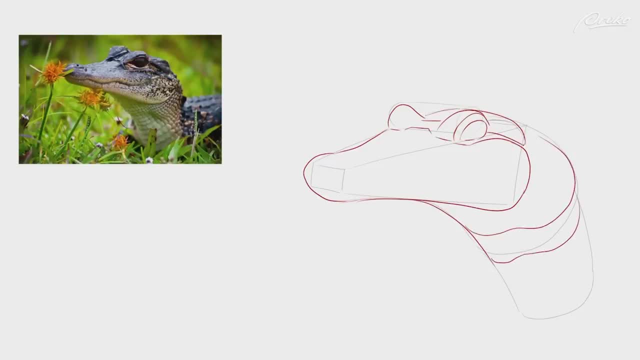 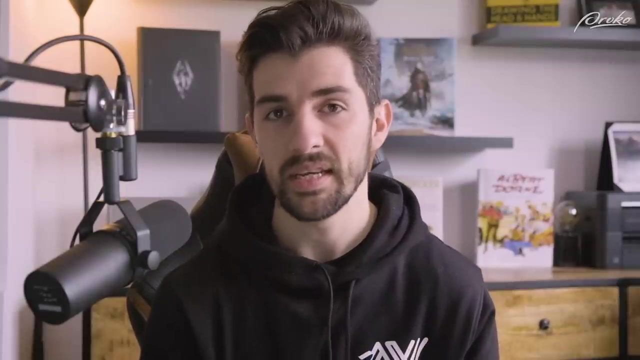 remember everything. but if you can mannequinize the things that you see and even not just make a very simple mannequin but also make complex mannequins with manipulated shapes, that's still a lot easier to understand. and i think a great example of this is an artist like kim young ji, where i don't believe that all he does is 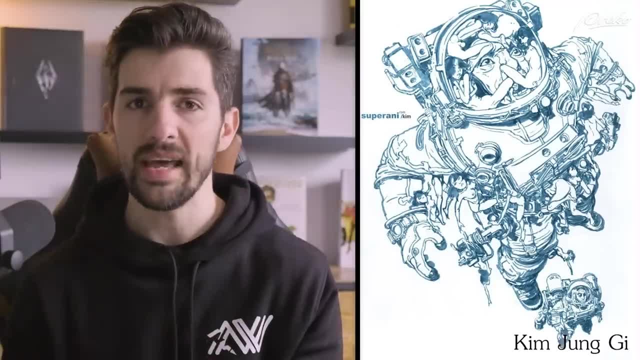 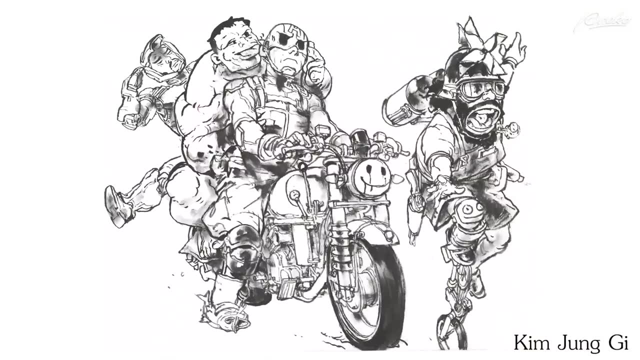 know, intrinsically know, the anatomy of every subject, but he does very much understand the complex, manipulated mannequin of the subjects that he makes, and he does very much understand the studies, and so that gives him the power to then, just you know, draw every subject in different. 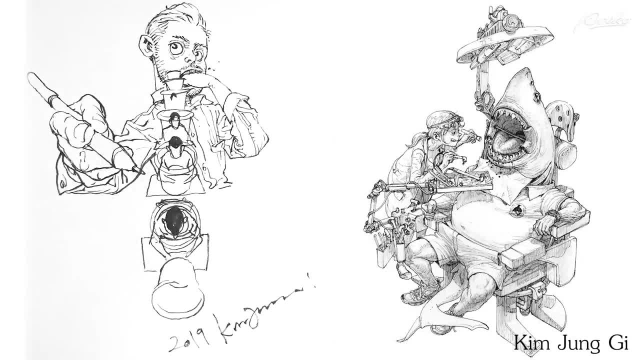 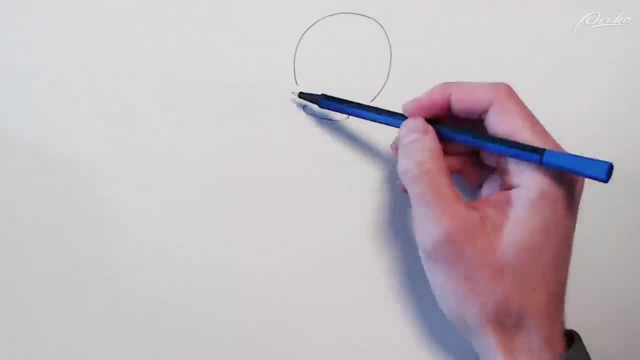 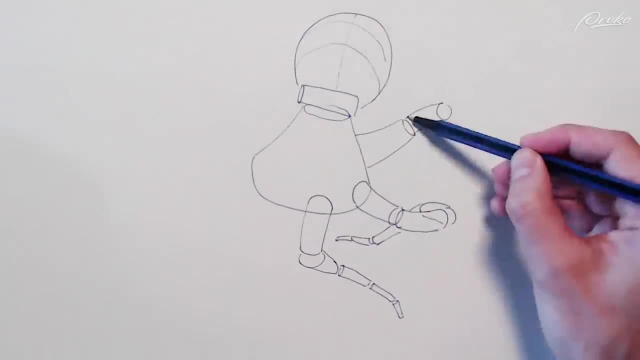 angles, from any, you know, in any perspective, because he has that power over the simple shapes which he can manipulate in space, and so, when it comes to observation, a really good exercise is to just look at. you know a multitude of of reference, especially things you want to specialize in, but 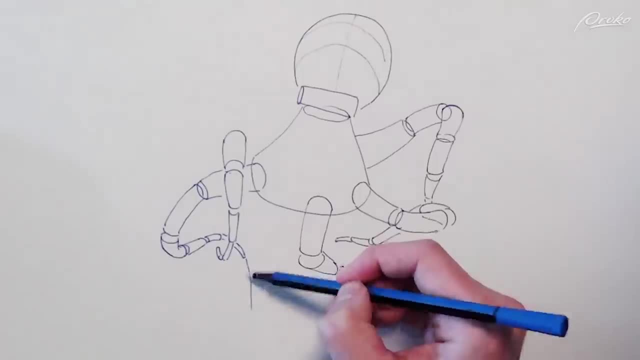 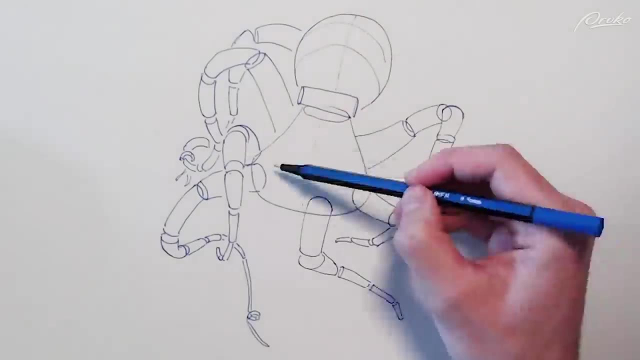 also things that that are outside of your comfort zone, because you know learning to draw things outside of your comfort zone will very, very much help you with things that interest you as well. again, looking at a lot of reference and then trying to mannequinize that reference using more. 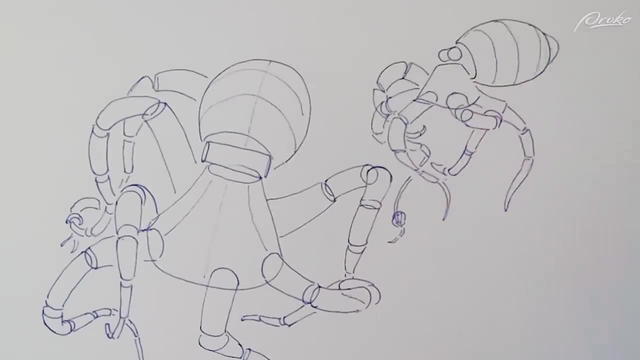 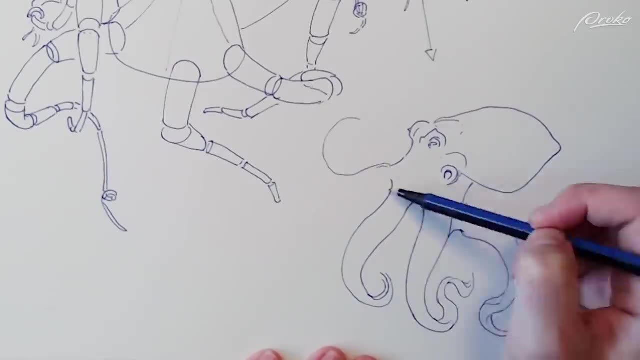 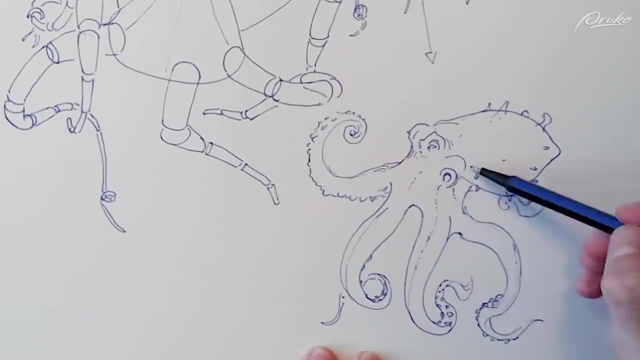 complex shapes and you can start off with a very basic shape, but then, you know, try to learn how to make a more complicated mannequin on those simple forms, right? so again, that's step one and step two. you look at the reference, you kind of try to figure out what simple shapes 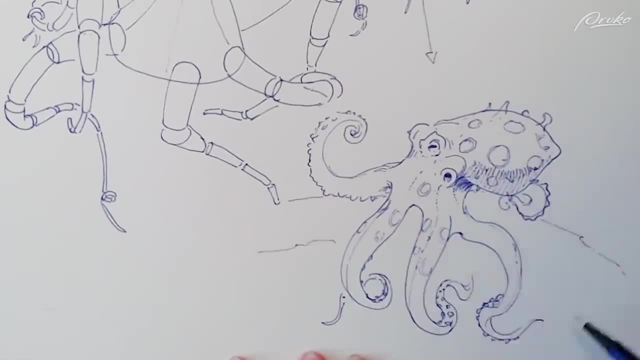 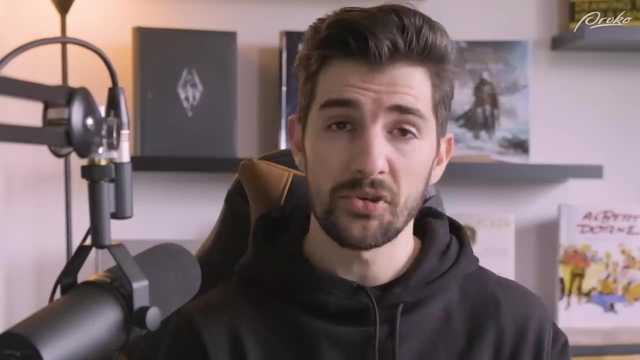 that reference is made up of, and then you try to figure out where those simple shapes are being manipulated. is there some form of contour manipulation going on, or there's some addition or subtraction? are some of the the simple shapes being twisted or bent? you know all these things, or? 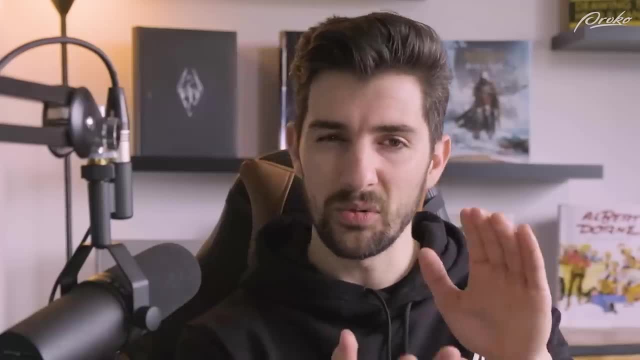 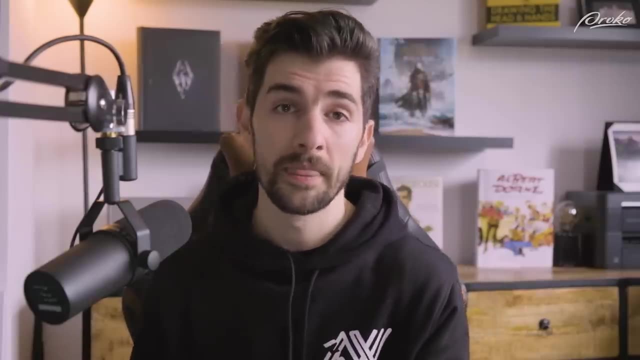 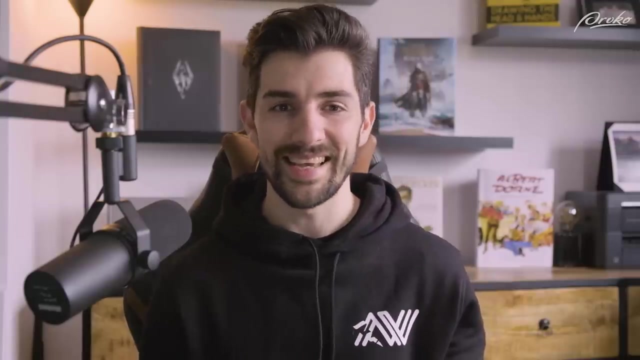 is it a combination of those? of course, all these things can help you understand that subject better. you know, if you have a good understanding of what you're looking at, then you can go into the next step, which is education. so, with education, this is exactly what the word implies- is that we're now we're trying to educate. 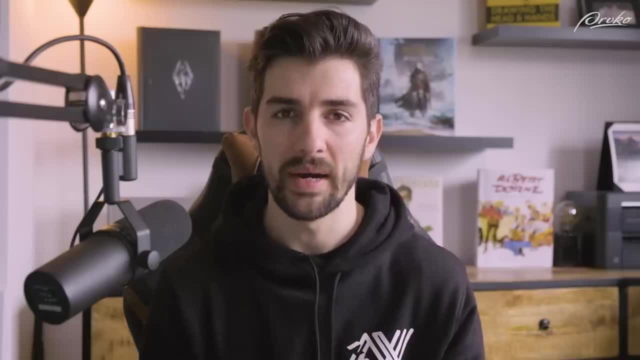 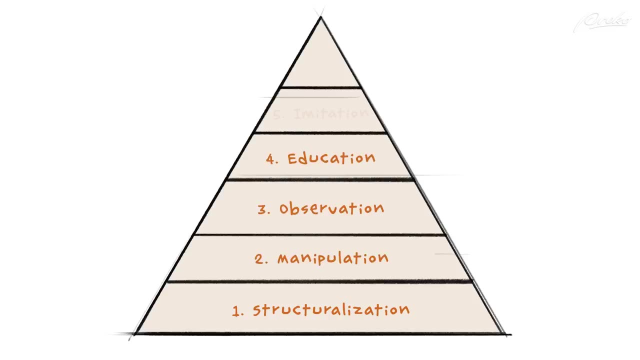 ourselves about the things we really want to know more about. so- and that's also a thing with these six steps- is that we kind of go from a broad sense to a more narrow sense, meaning that from step one, step two, step three, this can be very general, this doesn't have to be your subject of interest per se. 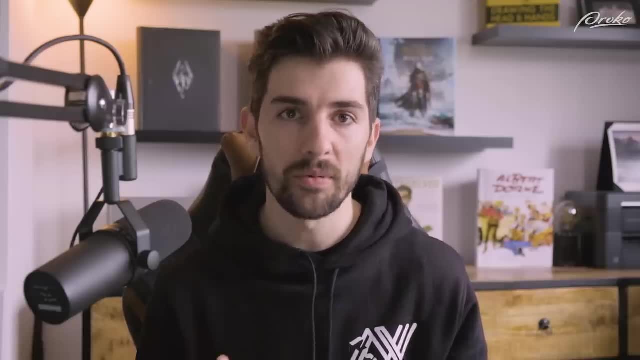 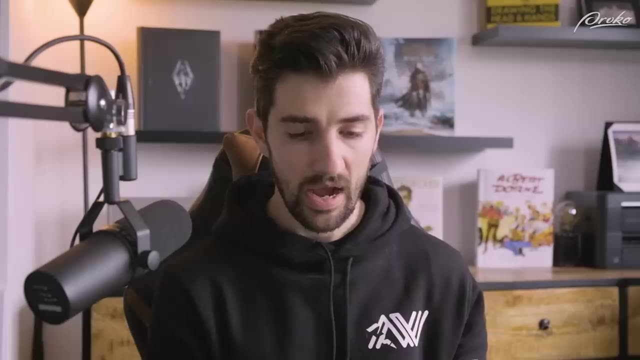 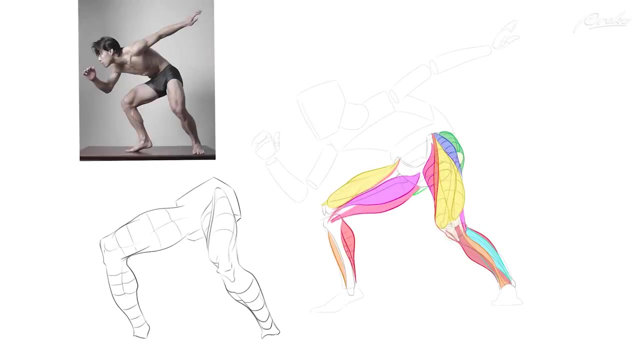 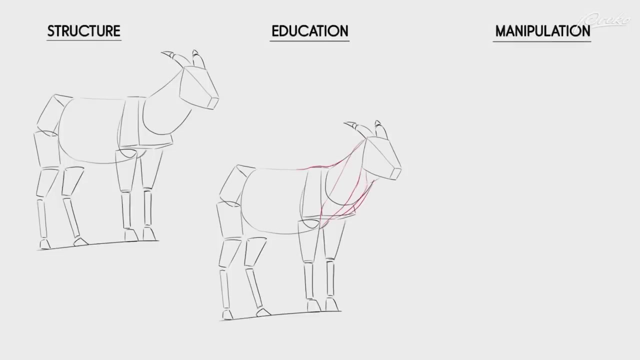 it's just something that will help you understand. you need some space, fine-tuning of study information, or would it visually☆ where you would like to learn more for the course? I guess it is like you know you have three levels right, and you have three different instruction levels and in this kind of sense, you start with the first. that's like you know what can I say when I post and I do moreAir 650, but then I'd like to start with another 278, 00 to do more Air´s 360 and things that interest me. so when I actually want to teach something, Dan needs to know what to learn more about the handcuffs or, for example, the basic personal informationhteach or stu immer a lot better, basically, drawing with structure. however, with education, we usually tend to want to learn more team work to learn about. 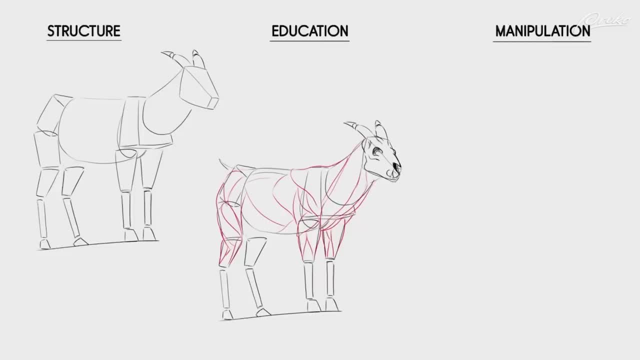 learning from observation with simple manipulated shapes. Now, the things that I'm learning about- for instance, the anatomy of the human figure or the anatomy of a certain animal- can better inform those manipulated shapes that I was constructing earlier. So that doesn't mean that we're completely reinventing. 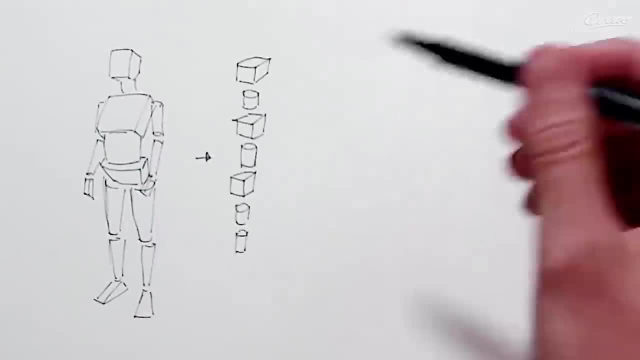 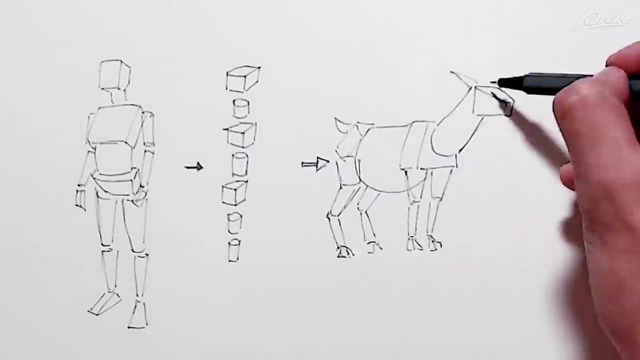 the way that we draw certain things just because we're now looking at its anatomy. No, it's actually. we can even better fine-tune the shapes that we were constructing before. Now we can have those shapes be informed by the anatomy that we're learning about. 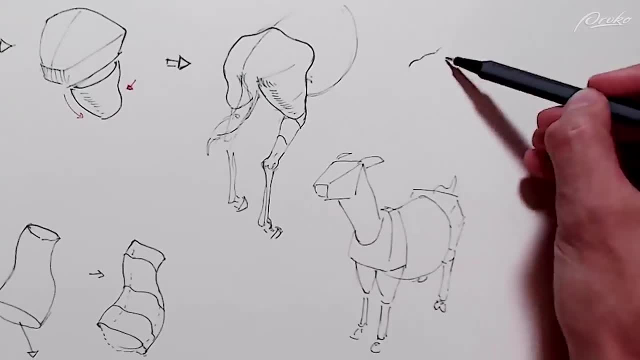 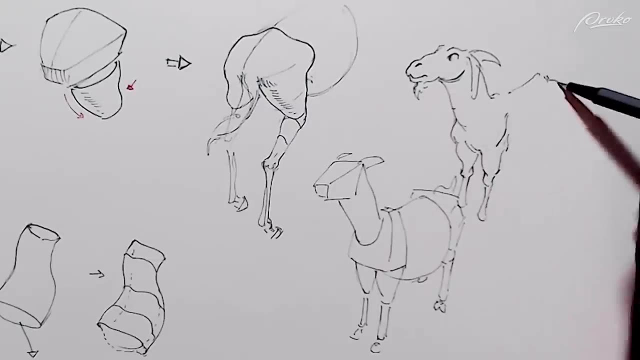 And that's why it's usually topics that are close to heart or things that really interest us, because now we're really going to fine-tune the things that we want to learn more about, just to become much better at designing them. So, when it comes to education, 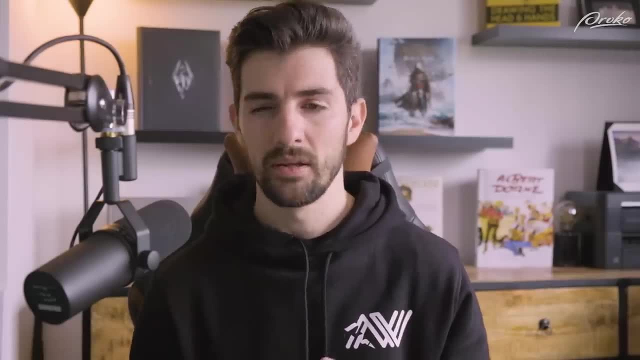 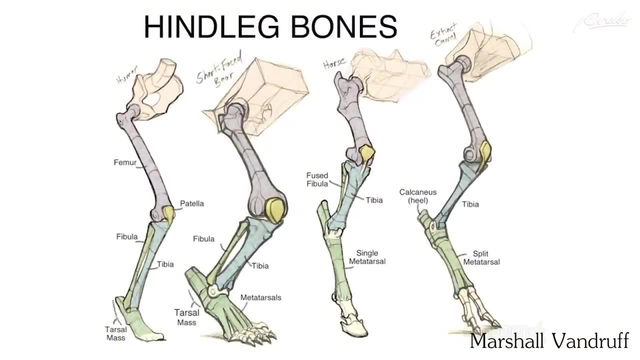 we, of course, pick the subjects that really interest us, learn about them intensively. the anatomy or the packaging of a vehicle. what makes up a vehicle? make a comparison between human anatomy and animal anatomy, especially if I like to draw horses. 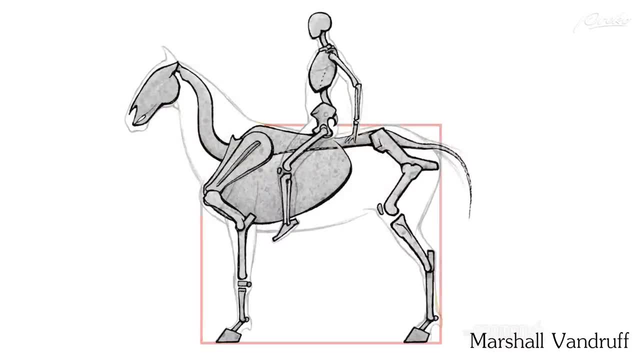 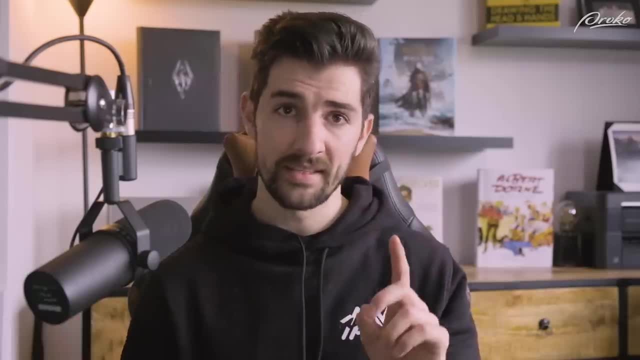 You know, if I'm a fantasy artist and I want to learn more about horses, I want to learn to draw dragons. You know, if you want to learn to draw dragons, you need to learn about bats, lizards, horses. Again, it's an amalgamation of a lot of elements. 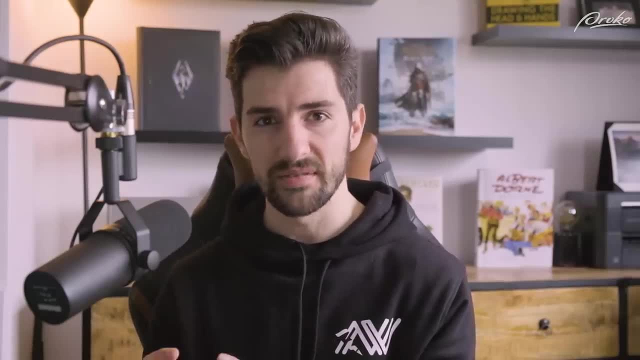 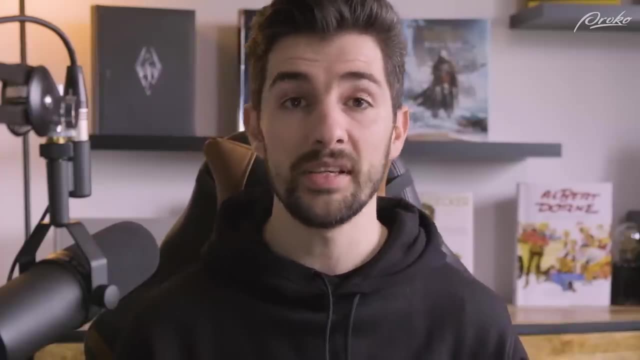 animals, but these are still specific subjects that you can learn intensively in order to help that better inform the complex shapes that you've already created, just to fine-tune your ideas and to become a better designer. Moving on into you know, step five. 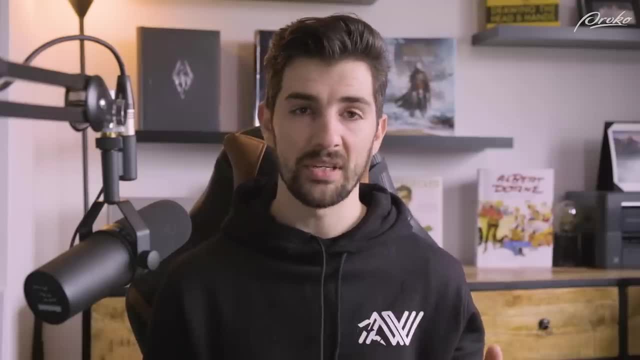 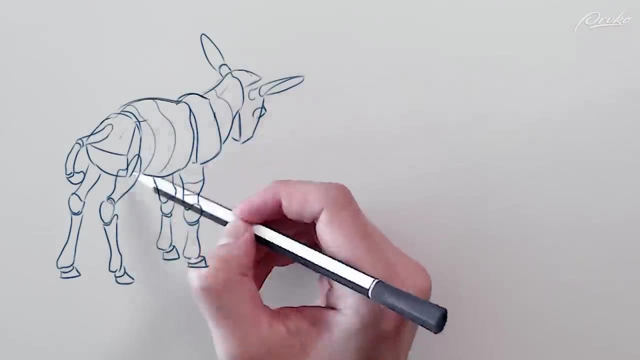 which is imitation. This is where we actually learn from our peers or the people that we look up to, to see how they're actually using all the principles that I've talked about to their advantage. So you know, I think it's really important. 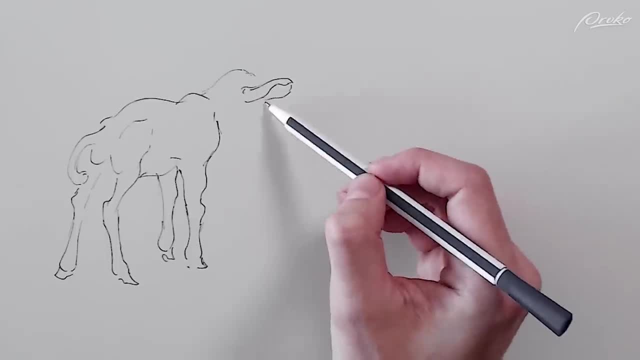 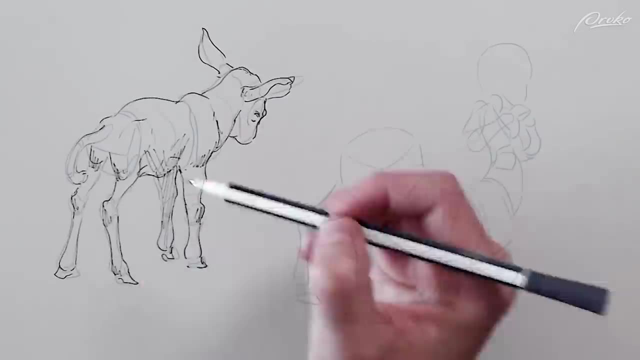 to take advantage, right? So I'm not saying that everyone that you look up to or every artist is using this sort of principle that I'm talking about, but you can definitely use these principles to analyze the artists that you look up to in order to use some of their shape language. 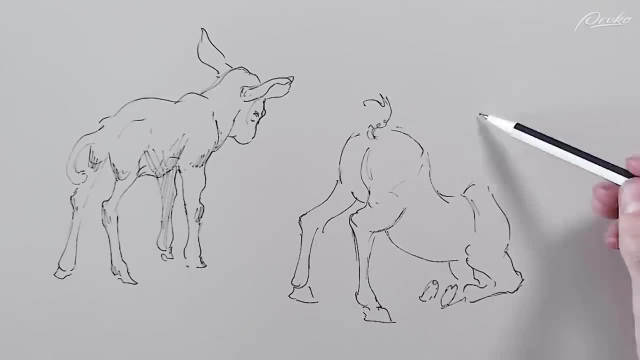 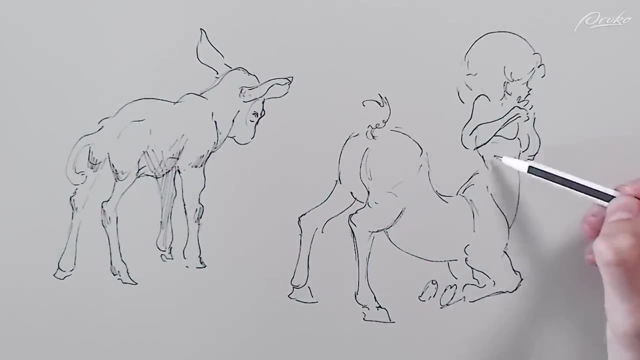 some of their ideation, some of you know, just their structuralization into your own designs, because that will, you know, make you a better artist. I think we sometimes tend to, you know, try and cultivate a style too fast. 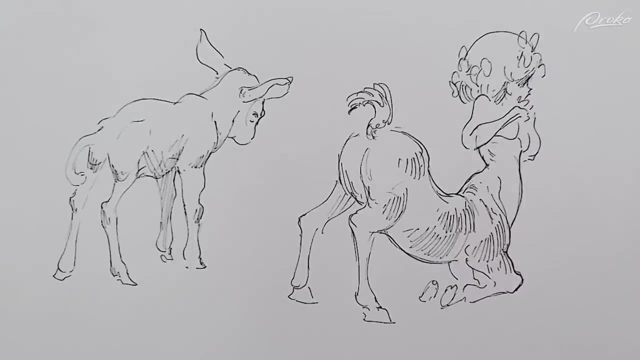 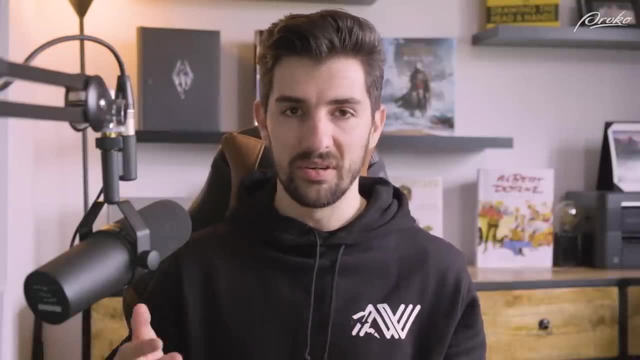 whereas there's nothing wrong with learning from the people you look up to. I would even say that you know, in order to cultivate our own style, we need to have an accumulation of people we look up to, and we need to have imitated those artists. 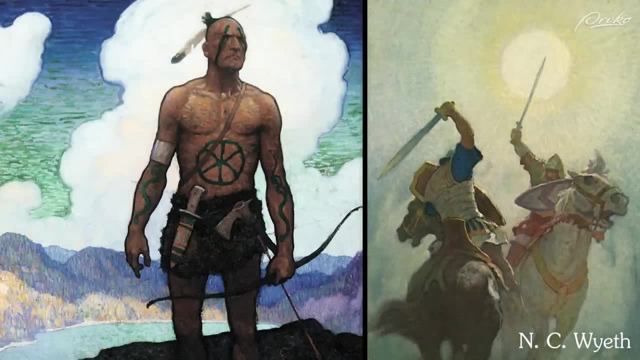 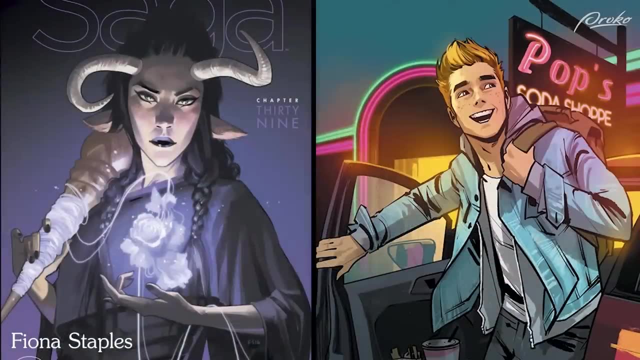 Of course we're not going to imitate one artist, because then we're just going to be a copycat of that artist. But if we can analyze all the artists that we look up to and we can, you know, pick a little bit of his or her design. 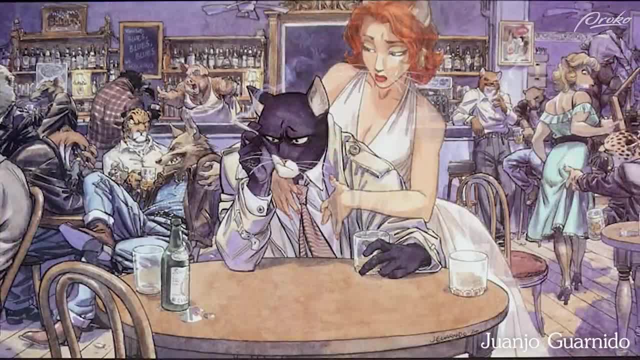 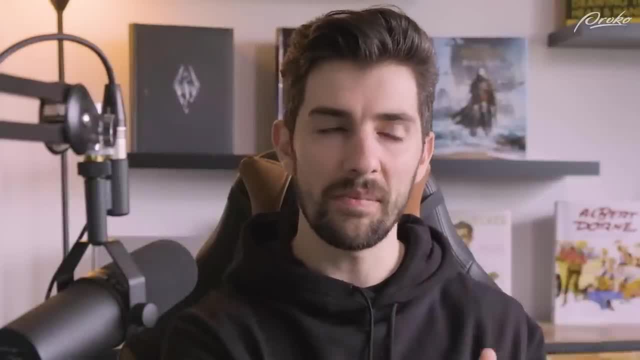 or you know the way they draw anatomy or the way they design certain vehicles or dragons or whatever. you can still analyze those. you know the structure and the shape manipulation that they're using and use that to your own advantage and use that into your own designs. 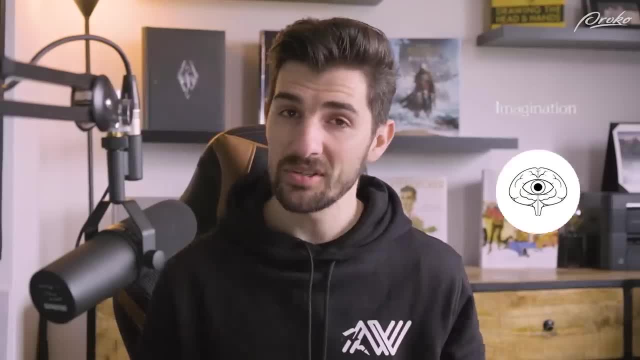 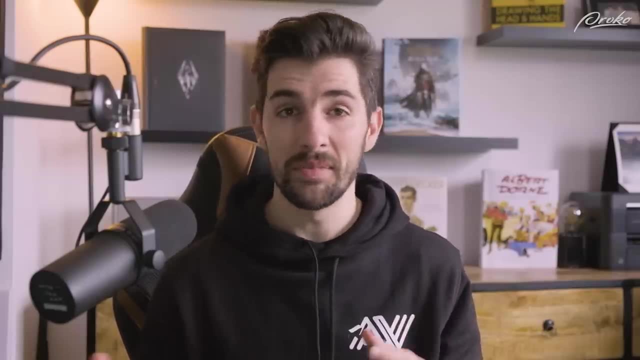 And then, finally, we arrive at the last step, which is, of course, imagination. So, as I said before once, we've gone through all the steps and we also imitated, or, you know, analyzed and studied our favorite artists. 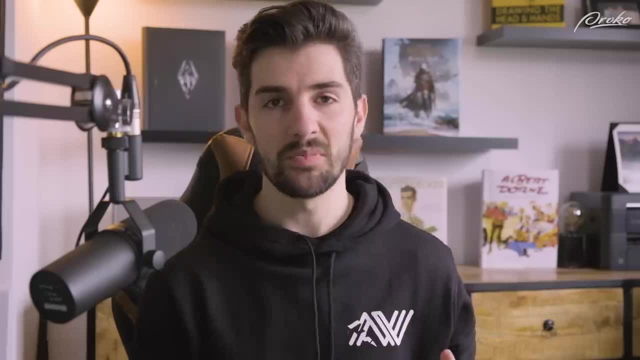 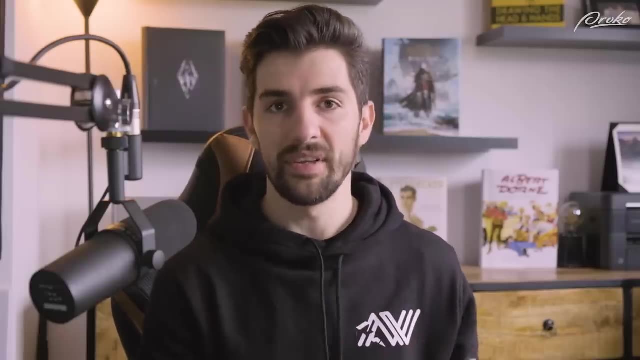 we can now try and come up with our own designs. Now, that doesn't mean that you cannot come up with your own designs without looking at other artists or, you know, even going through this process, but it will definitely help you or inform you to create better designs. 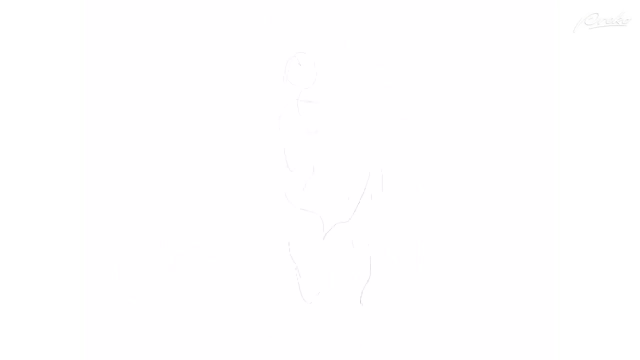 So when you've cultivated a vast library of mannequins with more complex shapes, manipulated shapes, and you've studied the artist, you've observed things from life, from reference, you've educated yourself about, you know anything that interests you. 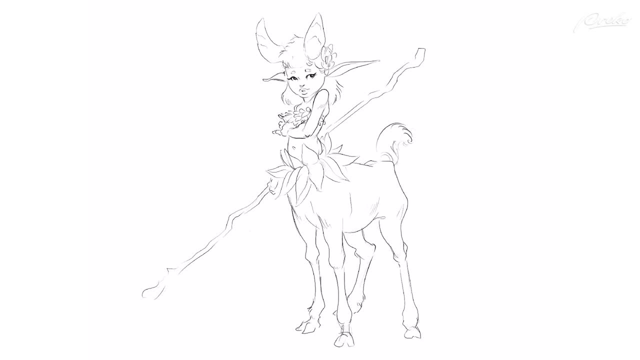 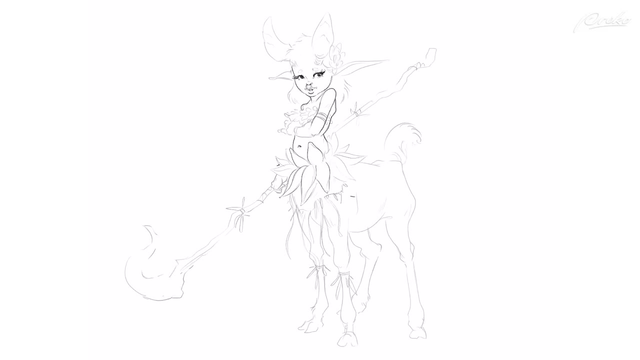 you know, this can all come together and you can create your own designs using all the knowledge that you've cultivated. So I think the most important part here is to just see where you are, because of course, there's a big difference between coming up with simple shapes. 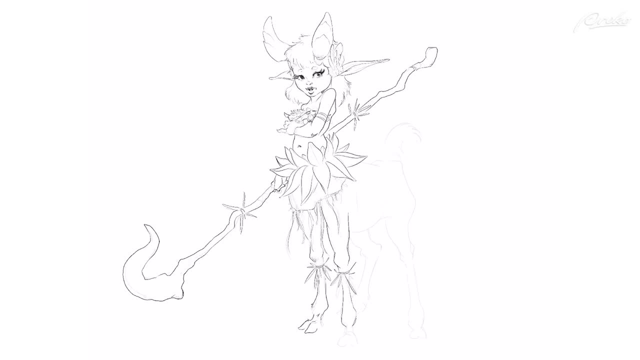 studying things that you can physically see, and even studying other artists, than it is to create something from scratch. Right, It's that old saying of you know, the fear of the blank canvas, which is, of course, it's very true. 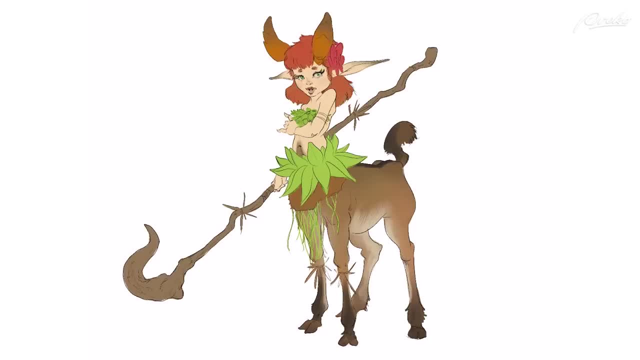 But now that you have all of these things in your tool bag, you can still start constructing ideas just from what you already know, and then see how far you can take this. The other thing that I also want to, you know, mention when it comes to drawing things from imagination: 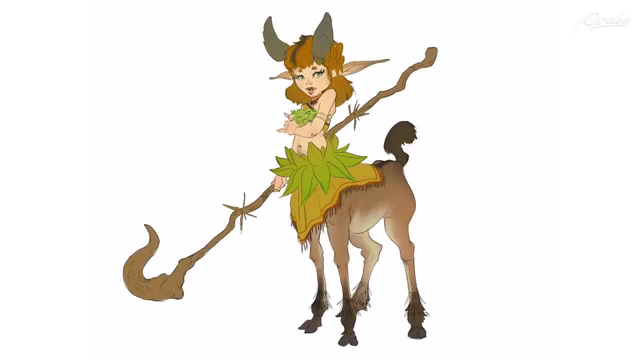 or at least from things that we know or from memory. it's not that straightforward process of going through structure, then observation, education and, you know, imitation. It's very much an intuitive process, so it also needs to be treated as one. 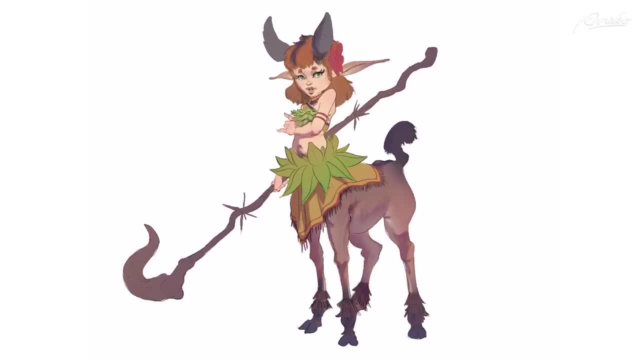 And I think what you need to be aware of when it comes to drawing things from imagination is that we kind of reverse engineer all the things that I've just been talking about, Meaning that you know, you've heard of the, the thumb nailing process when it comes to being a concept artist, 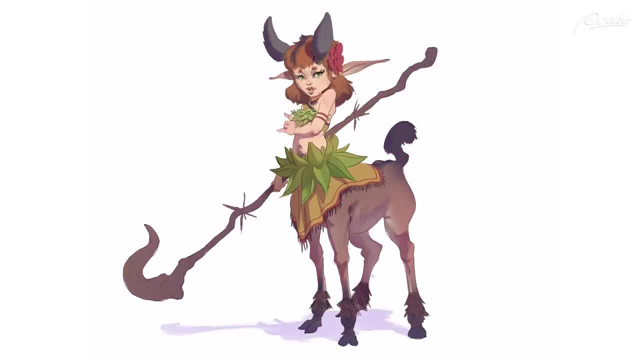 which is a very necessary process sometimes, Because that's actually What we do as concept artists is we try to solidify the abstract Meaning, that we create interesting shapes to the interesting silhouettes, you know, that have a certain rhythm flow. 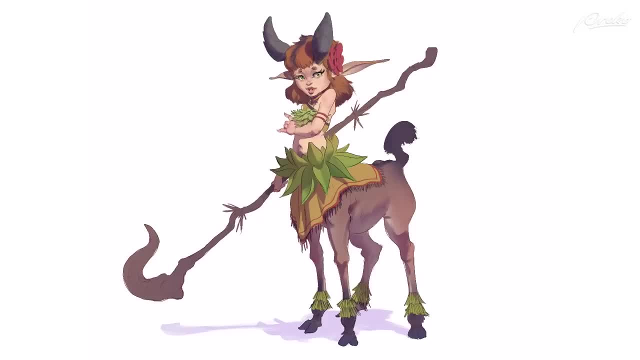 a certain cool design And then we try to structuralize these silhouettes or abstractions to create something that is usable and tangible in a game or a movie or whatever. So what we tend to do is we tend to make something that is abstractly appealing. 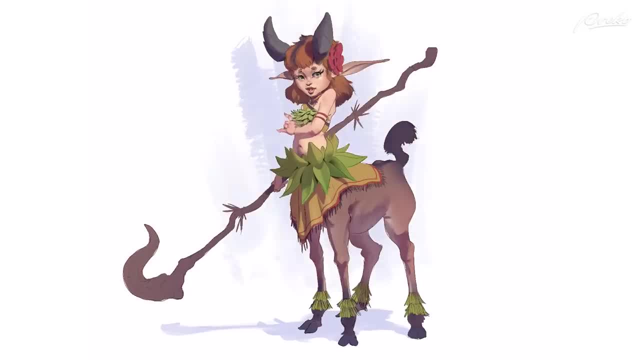 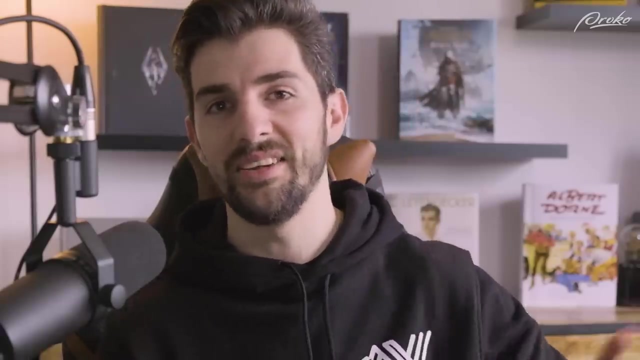 but then we reverse engineer a lot of the steps that I've been talking about to solidify that abstraction, to make it, you know, actually tangible and usable and believable. So drawing from imagination does require a whole lot of different set of skills. that you know. 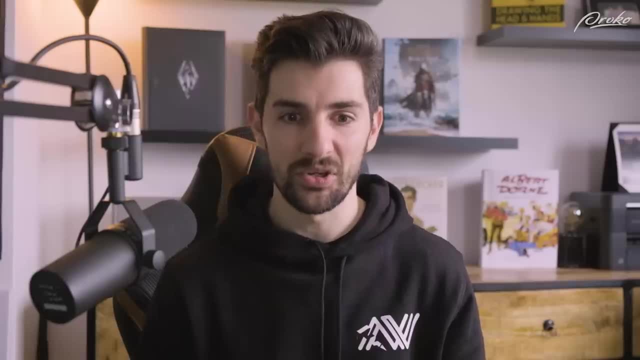 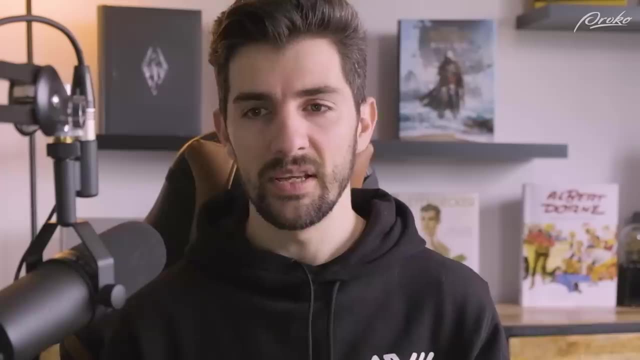 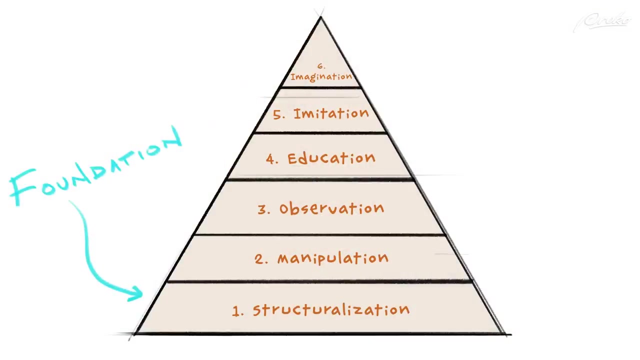 I haven't covered in this video, But I just wanted to kind of emphasize the importance of structure when it comes to drawing and painting. It's something that doesn't, or shouldn't, be overlooked. Especially the second step, when it comes to shape manipulation, I feel is a very important one. 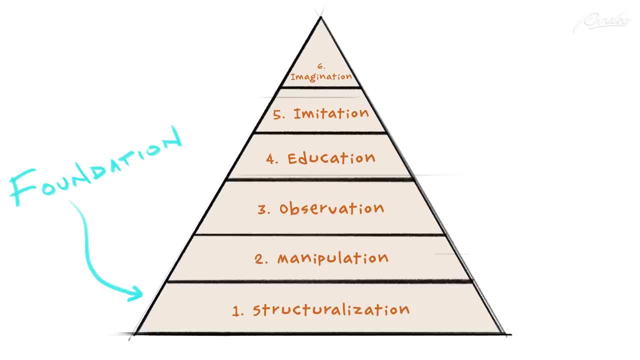 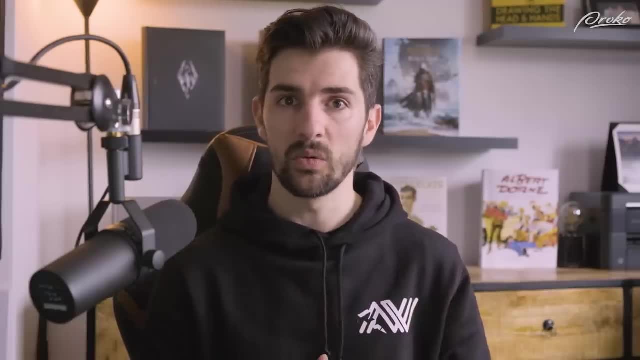 which is often overlooked, Even when it comes to design. I did a workshop once on product design and I asked the woman in question that was giving the workshop, which is a very, very famous product designer: how can I become a better designer? 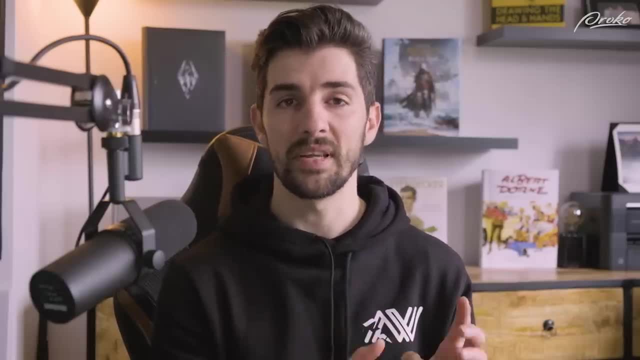 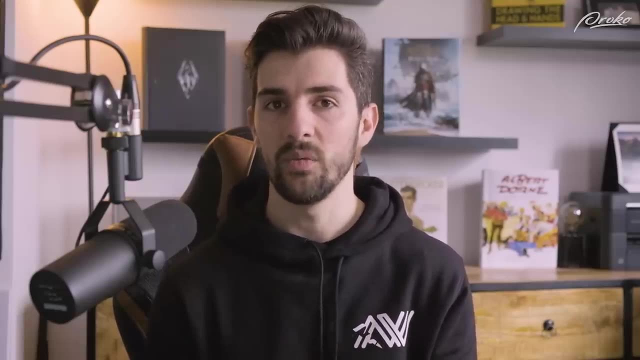 And she told me: have you ever tried to make simple shapes like cylinders and boxes look interesting? Which completely caught me off guard because I never thought of it that way. But she told me, like, if you cannot even make a simple shape look interesting, 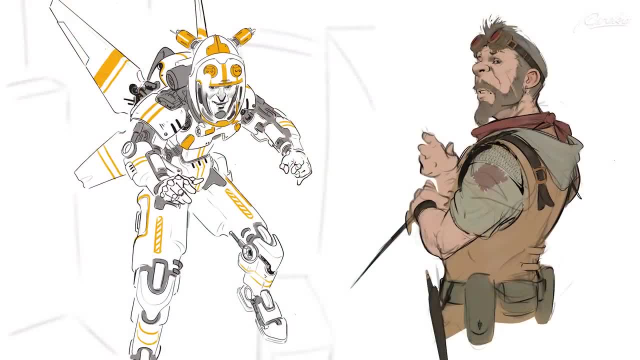 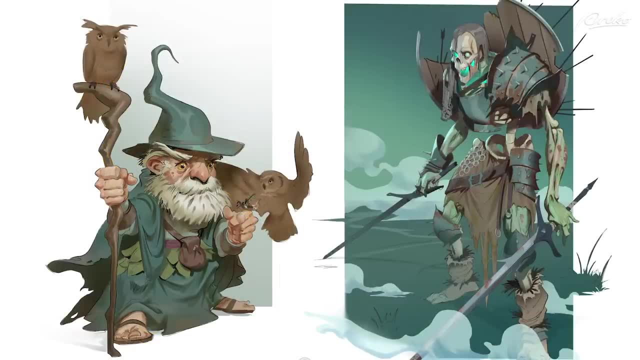 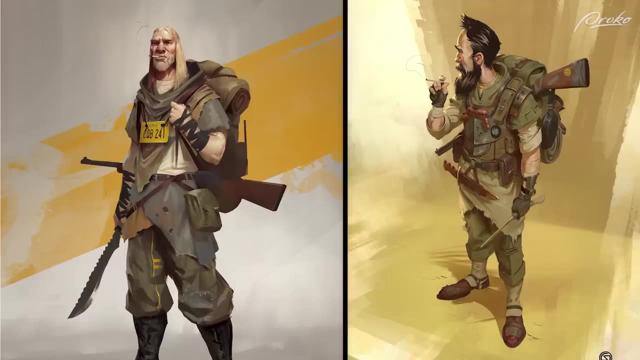 why bother making complex designs right, And there's a lot of truth to that. And I think if you try to first learn to draw the simple shapes, the structure, learn to you know, create spatial awareness, learn about the different perspectives. 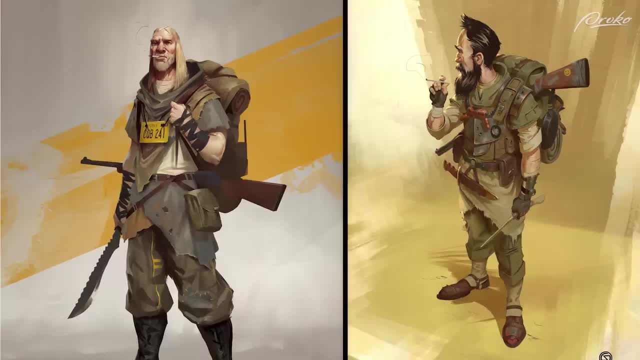 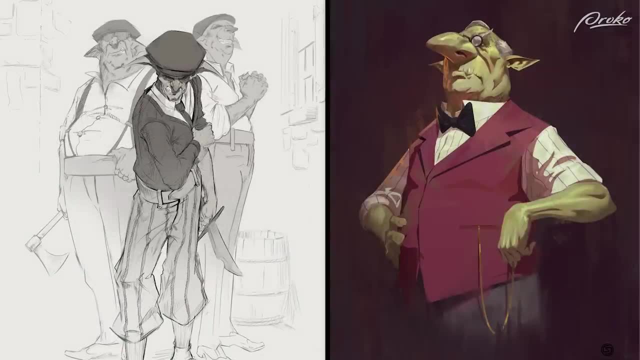 you know and things like that, but then try to manipulate those simple shapes with the things that I've been talking about and a lot of other things that other artists have already mentioned in the past, just to be able to focus on the task at hand. 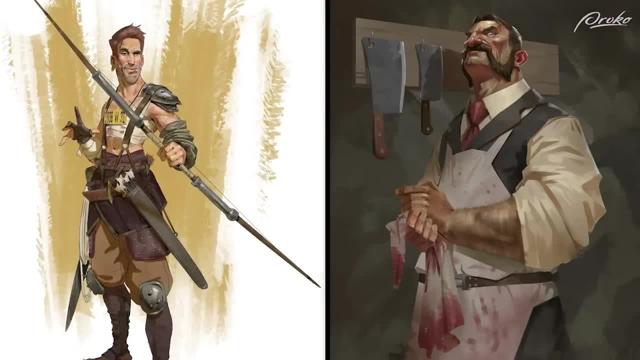 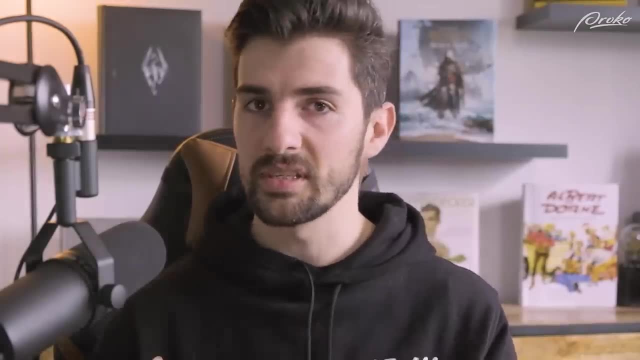 And if you can create that convincingly then you'll have a lot more confidence. moving into more complex subjects Like humans, character designs, creature designs- you know drawing animals, even drawing from life, If you want to be a fine artist that wants to. 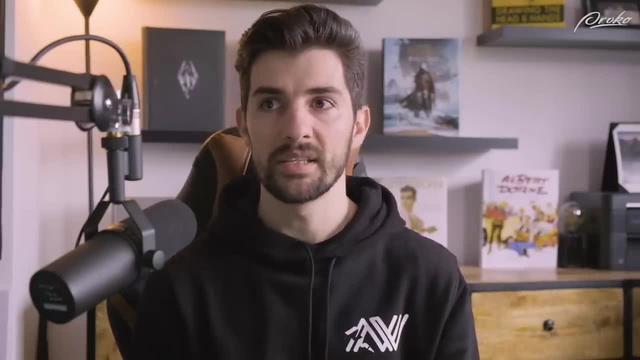 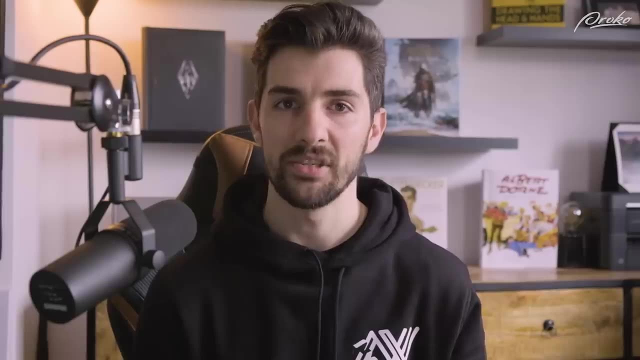 learn how to paint horses right. It still very much pays off to know the more complex mannequins and be able to do things from imagination, even if you're using reference. Sometimes, when you're using reference, you're still looking at a 2D image. 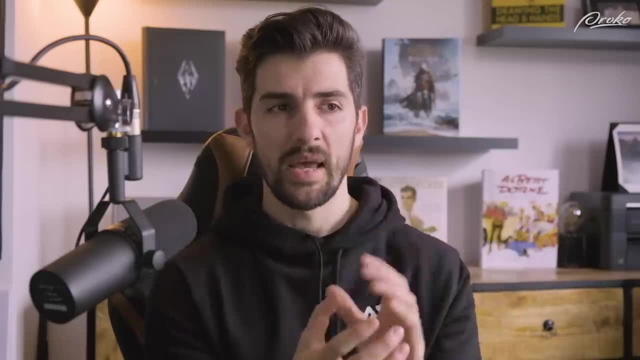 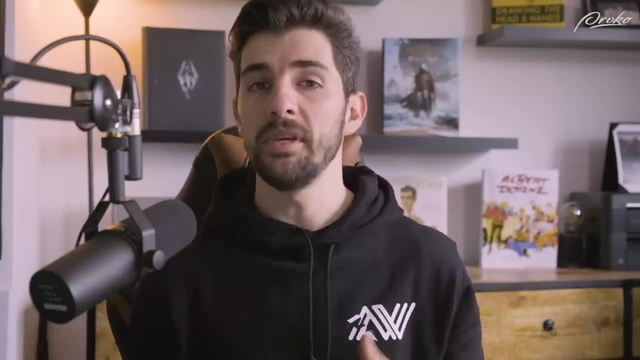 So if you can analyze a reference and understand its more complex shapes, and maybe you know, mannequinize it in your head, it will become easier to then paint at or, you know, alter certain things that you don't want to see in your final painting. 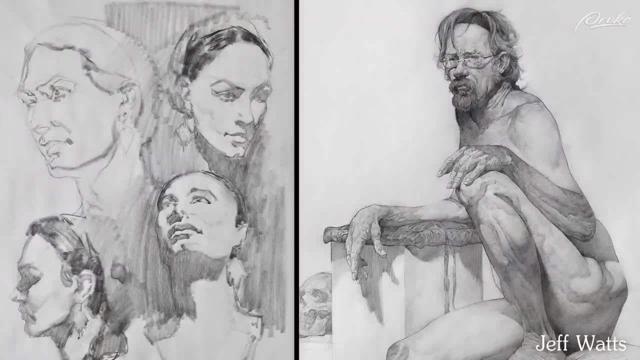 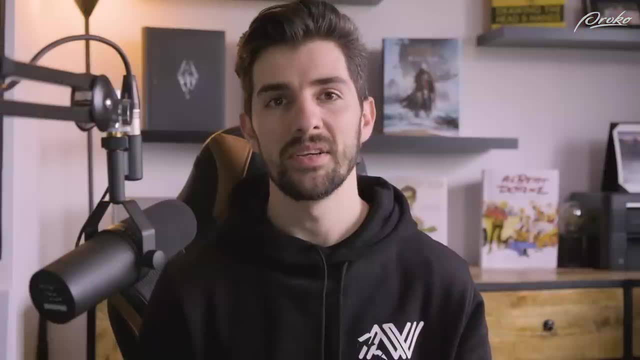 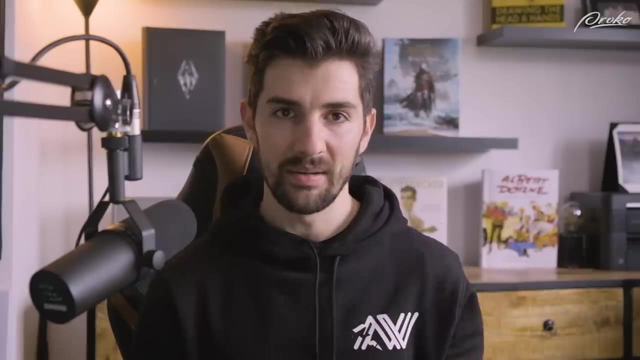 I think Jeffrey Watts famously said once: try to manipulate your reference and not be manipulated by your reference, And I think that's a great quote, because it actually means that you're you need to understand the subjects that you're drawing or painting instead of being manipulated by what you see. 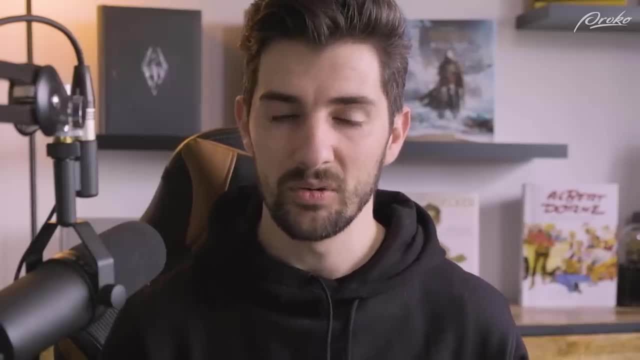 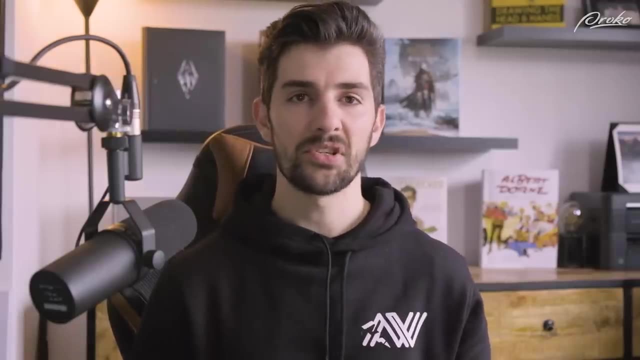 And then, lastly, what I still want to, you know, briefly say, is that structure isn't only, you know, putting things on paper or on canvas, It's also about having structure in your artistic training. So the only way to get better is to have